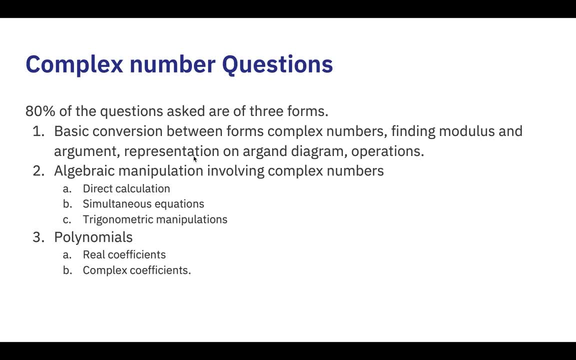 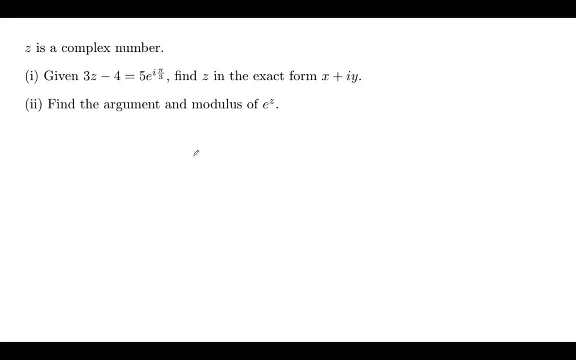 with both real and complex coefficients, right? So we're going to dive right in to the first type of question on basic operations. Okay so, given 3z minus 4, when z is a complex number equals to 5. e to the power of i times pi over 3, find z in the exact form: x plus iy And part 2. 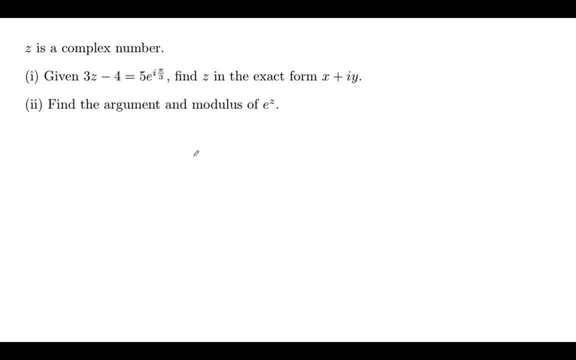 asks us to find the argument and modulus of e to the power of z right. So to do these type of questions, you need to be very comfortable with how to convert between the forms, the different forms: rectangular form, polar form and exponential form of complex numbers. Okay so, 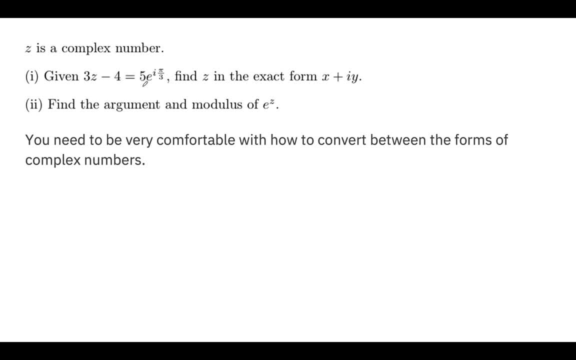 to do this question. the first thing we want to do is we want to convert this thing over here into rectangular form, right? So we first convert it to polar form by writing it as so: 5e right. This over here is: 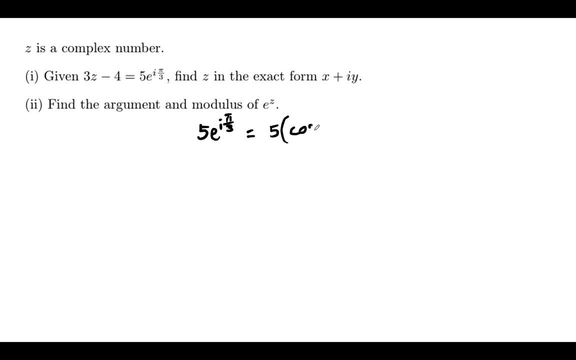 equals to 5 times cosine pi over 3, plus i sine pi over 3.. All right. next we realize that, okay, cosine pi over 3 is equals to half, so this is 5 over 2.. And sine pi over 3 is equals to square root 3 over 2.. So we get something like this, right, And now a simple rearrangement will allow us to obtain: z is equals to 13 over 6, plus 5 root 3 over 6, right, So we've expressed z in a rectangular form, as desired. 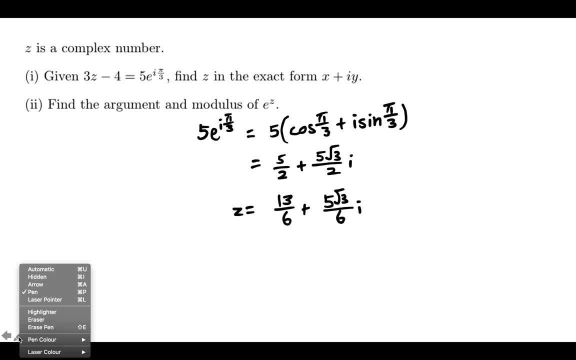 Now the next part asks us to find the argument and modulus of e to the power of z. So how we do this is we simply write out e to the power of z as follows: We write z in its rectangular form from the first part, right? So we get this, And then we can split up the exponents here as such. 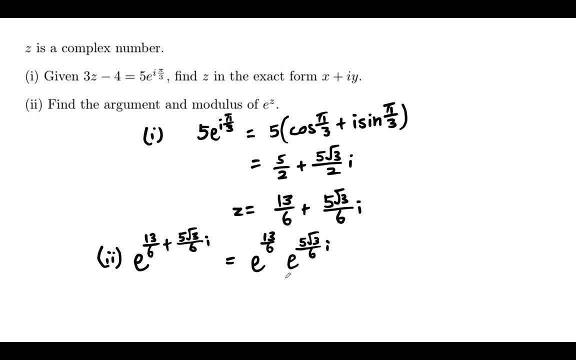 Right, so this is actually equals to our r, is equals to our modulus And this term over here- 5 root 3 over 6, is equals to our argument. So we write it as follows: This equals to e to the power of 13 over 6.. And argument of e to the z is equals to 5 root 3 over 6.. 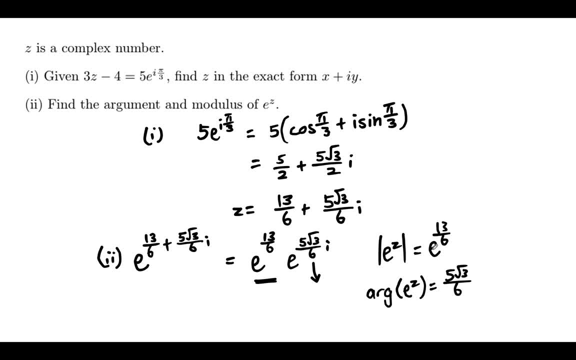 Now, before you write this down as your final answer, you have to make sure that this value is in between minus pi and pi, right, Okay, but here it is roughly equals to about- I think about- 1.44.. Right, so this is our final answer for argument. 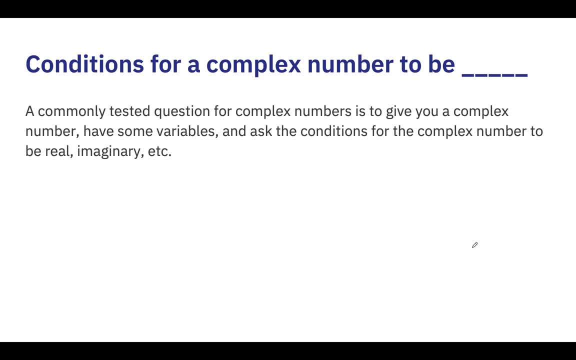 Right. so the next type of question that you like to test is the conditions for the complex number to be real or imaginary, etc. etc. A commonly tested example would look something like this: So let w equals to 1 plus square root 3i and z equals to minus 4e, to the power of i times minus pi over 6.. 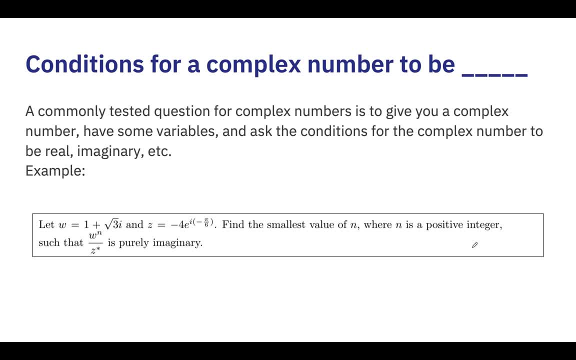 Find the smallest value of n where n is a positive integer, such that w to the n over the conjugate of z is purely imaginary, Right? so upon first glance at this question we realize there's a lot going on, right? So one of the first problems we have is that z is not written. 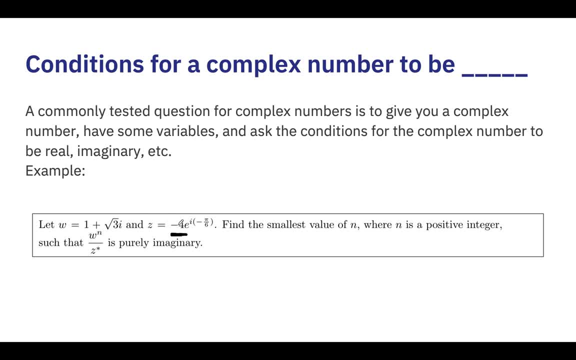 It's written in proper exponential form because its modulus is negative. This doesn't mean, however, that z isn't a complex number. It still is a complex number. We just have to find out how to make the modulus a positive value, right. 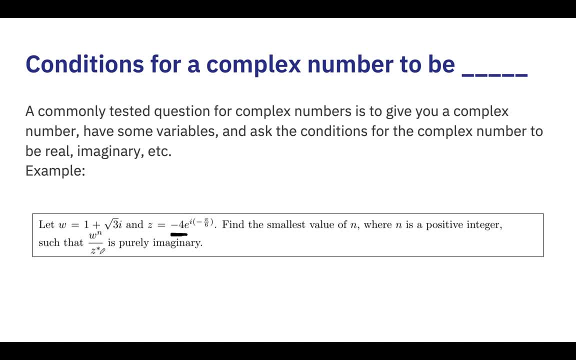 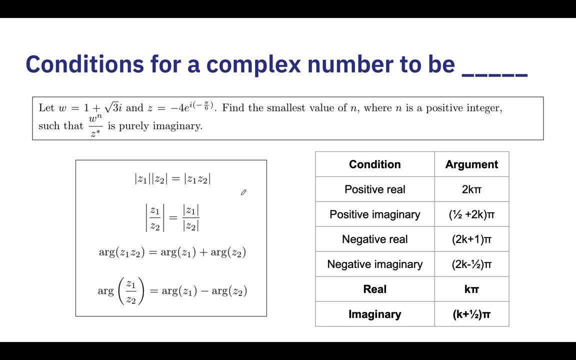 And they want the conjugate of z here instead of just z itself, And they want to raise this w, written in rectangular form, to the power of n, And they want it to be purely imaginary. So in order to do this question, we'll need a few of these properties that we've learned about: modulus and argument. 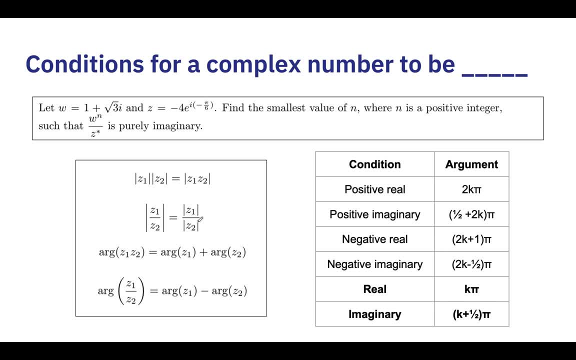 So the product and the division of modulus. you can split it up like this And argument becomes addition and subtraction. Okay, so I want to bring your attention to these last two conditions over here, In order for a complex number to be completely real, which means the coefficient in front of the i is 0,. 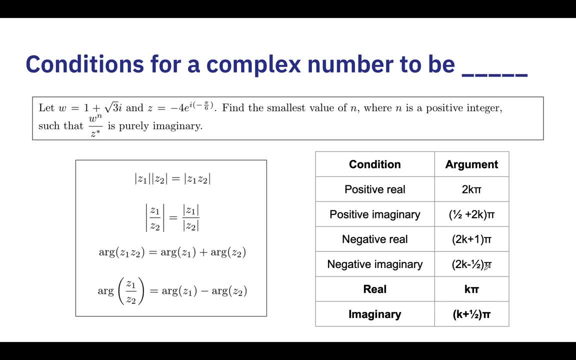 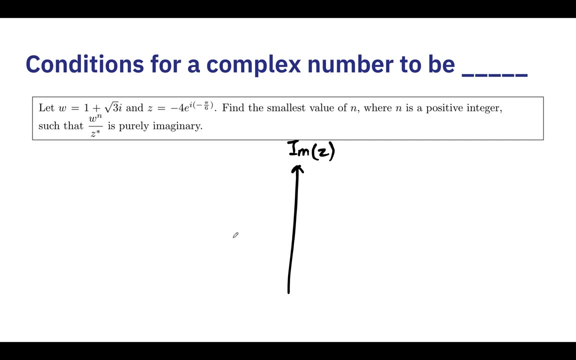 so there's no imaginary part. the argument must be equal to k, pi. Okay, why is this so? So, if you think about it, if we draw the Argand diagram right, Let's say we have a random imaginary number, complex number z, with real and imaginary parts. 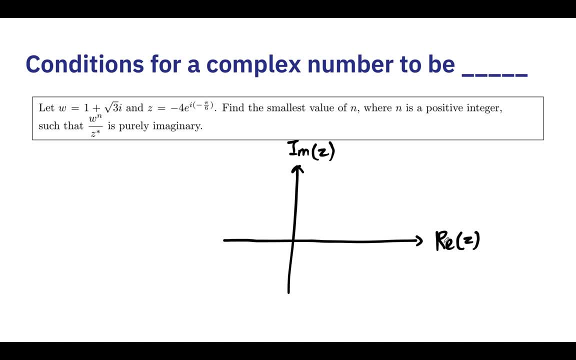 So the Argand diagram dictates that the horizontal axis is the real axis and the vertical axis is the imaginary axis. Okay, so in order for a number to be completely real, it must lie along this axis, right? so remember, our argument starts from the positive real axis. so if we 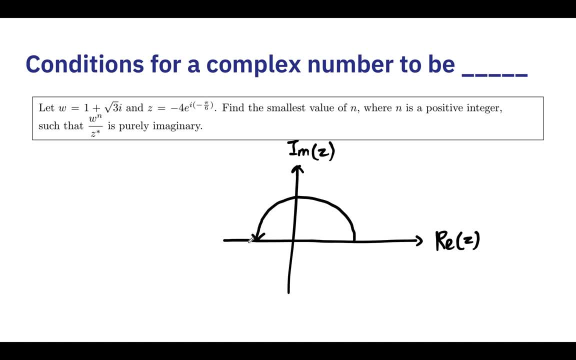 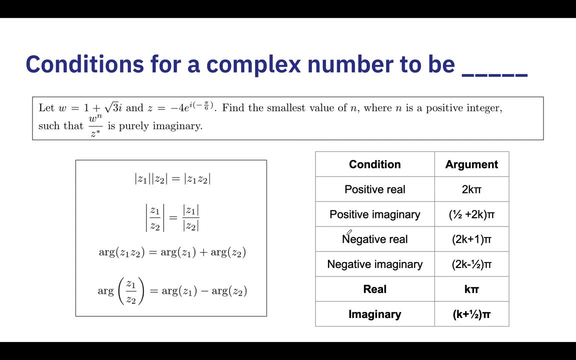 rotate it: pi degrees, pi radian. sorry, we'll get to a point on this axis as well. so this is pi and I rotate another pi, 2 pi, we get back to this line, and then 3 pi, 4 pi, etc. etc. so we see that the argument for a complex number to be 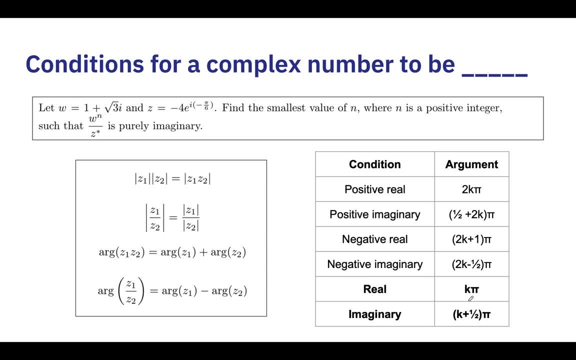 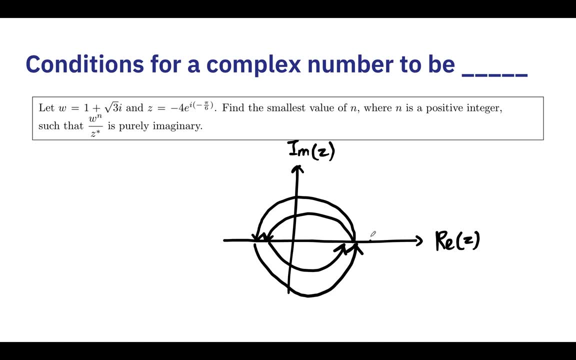 completely real is equals to k pi. so the multiple of pi, if it's imaginary, means it instead of making these kinds of full revolutions, it starts off by making a half revolution. right, this is pi over 2 and it lies completely on the imaginary axis, and then we continue to rotate it by another pi, so this is 3 over. 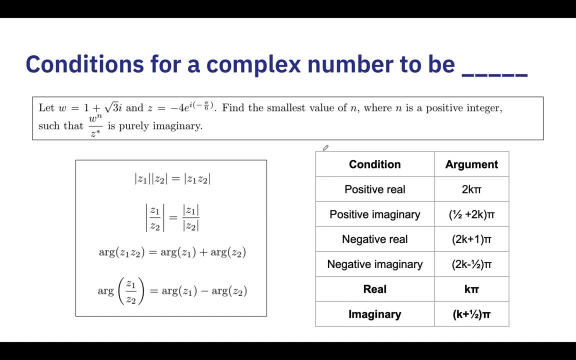 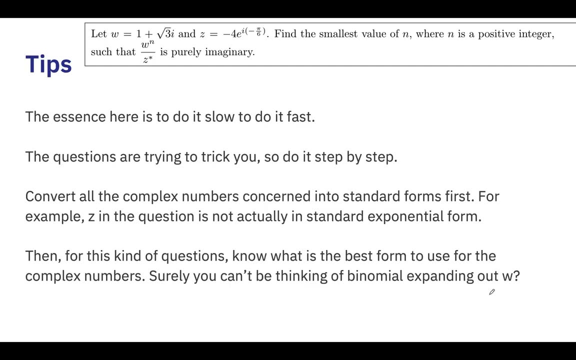 2 pi, and then 5 over 2 pi, so on, so forth. right, so these are very important and you should remember them as they'll be helpful. you in writing this question, in writing the condition in a mathematical form in order for us to solve the question. okay, so first we want to convert all the 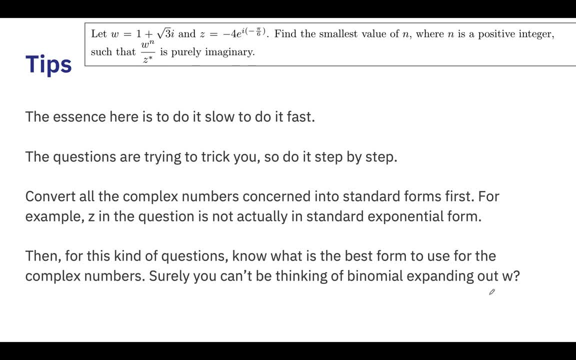 complex numbers concerned into standard forms first right. so, as mentioned before, z in the question is not actually in standard exponential form and for W they want to raise it to the power of n right and if we try and use the rectangular version of W it's going to be very 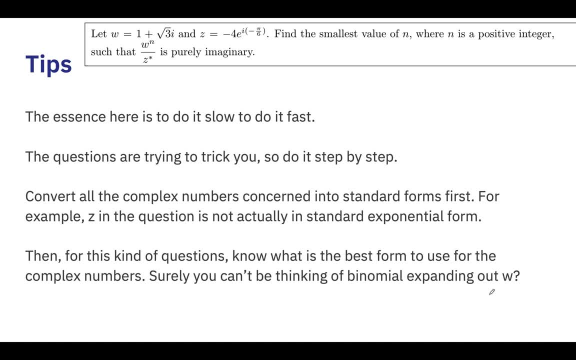 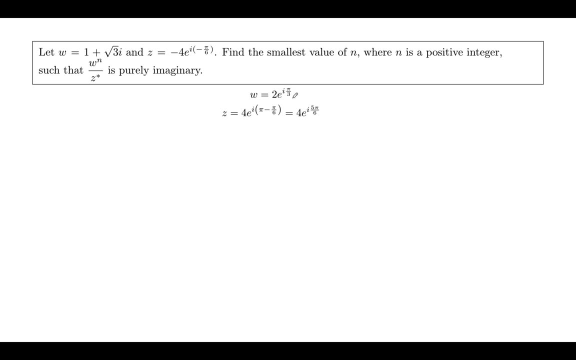 difficult to raise it to the power of n, as we have to turn to binomial Shooter, which is certainly not the case and not what we want to do when it comes to complex number questions. okay, so first we convert W over here in two exponential form, and as for z, we have to convert the minus 4 to 4. so I want to. 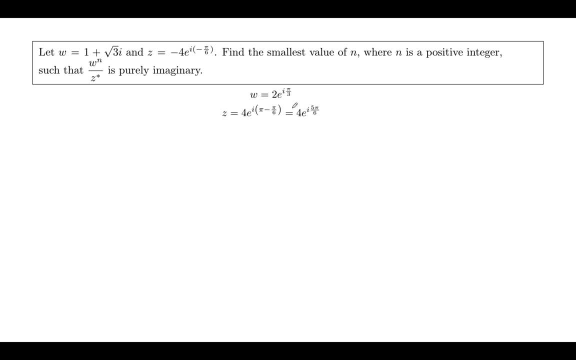 illustrate how to convert z into this proper form over here where the modulus is positive, right. so we first write this out in polar form and we got this here and i'm going to illustrate this: how to convert z into this proper form over here where the modulus is positive, right. so we first write this out in polar form as the formula here: the coordinate of n and z as we convert in☆ Sydney. and here we have twoились and we have two things to solve Uz with, but unos, in this case a. so if you've been solving z, ask for n and z Inclusive n. 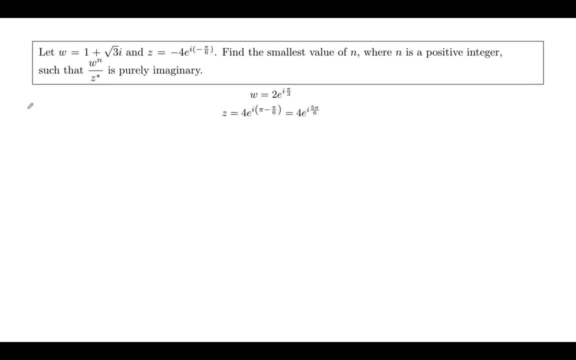 we write: sorry, z equals to minus 4, cosine of minus pi over 6 plus i sine minus pi over 6, right? and then we try and make this modulus positive, so we remove the negative sign and bring it inside. so it looks like this: 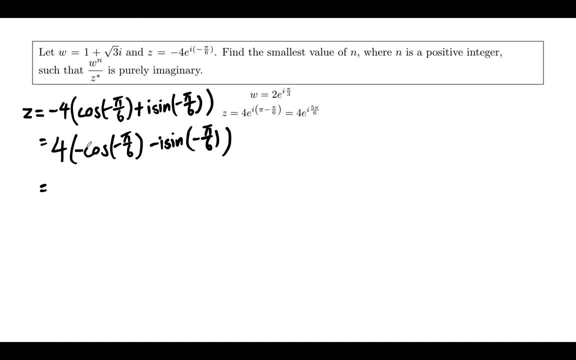 right, okay, so we realize this isn't really in the form that we we are looking for. right, because there's a slight issue, because instead of cosine plus i sine, we have these negative signs here that we, we don't really want. so what we're going to do is we're going to make 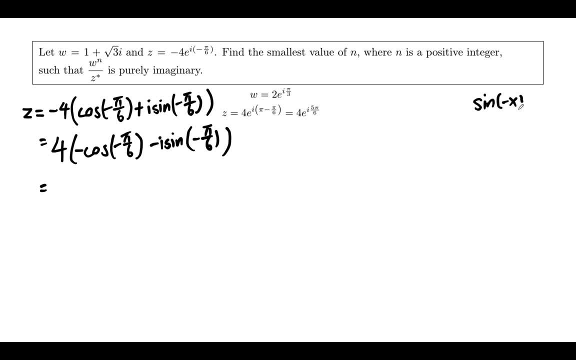 use of these two properties, sine of negative x equals to minus sine x, and cosine of minus x equals to cosine x. so using these two properties, we can write it like this: so the minus pi over 6 simply becomes pi over 6, and the minus in the sine comes out, so it becomes a plus. 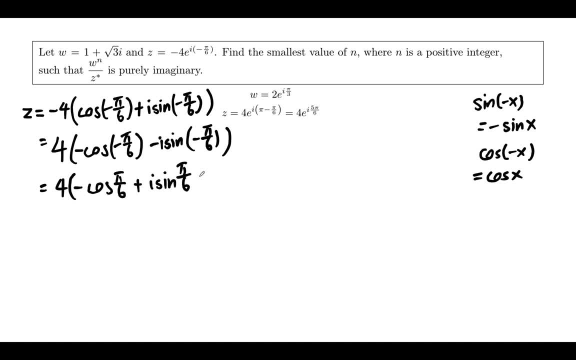 right. so, as we can see, we've managed to get rid of one of those pesky negative signs, but we still have this other one to handle here, right? so the next property we're going to introduce is to do with pi minus x, so sine of x is actually the same as sine of x. 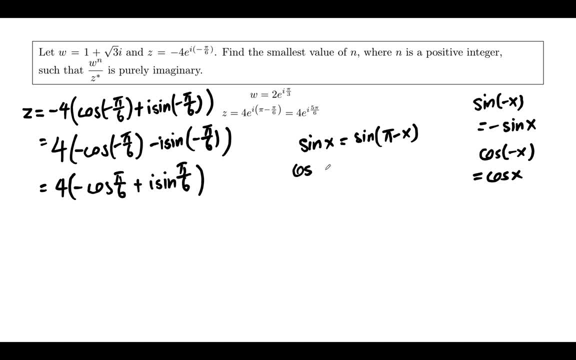 so it's psi over six. because so if we replace the angle inside pi here, then we definitely change the minimum angle inside to pi minus pi over 6, because if we do that then it will go back to 5 and we have a point halves negative. so its always length we don't want to have. 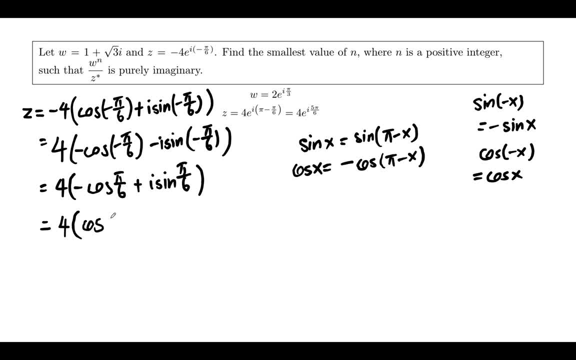 pi minus X, but we can't change that, which means that this shall go back to minus pi, minus pi over 6. so we can see, by simply replacing the angle inside over 5, this is the sine. that will be minus pi over 6 in the sido problems. 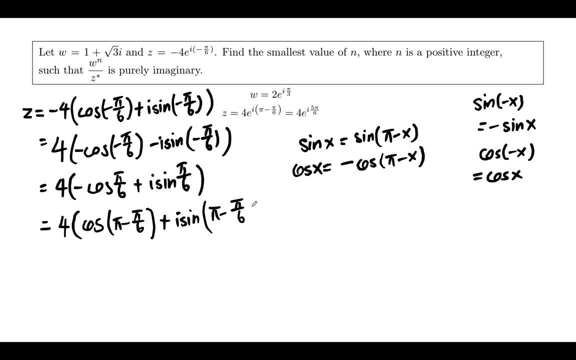 wouldn't change this sign over here, and we have it in our desired polar form. so we have cosine 5 pi over 6 plus i sine 5 pi over 6, right. and then we can we have the argument 5 pi over 6 in the desired form. so remember the minus pi over 6. 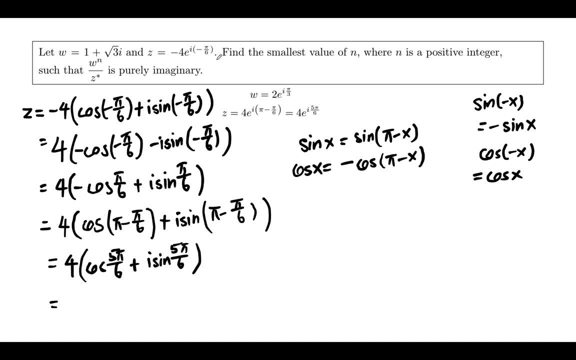 here isn't actually the argument. we have to convert it into the proper standard form before we can see what the true argument is, and then we can write it in exponential form, so it becomes like this: okay, so that is how we convert this non-standard form into the more standard exponential form. all right, so take some. 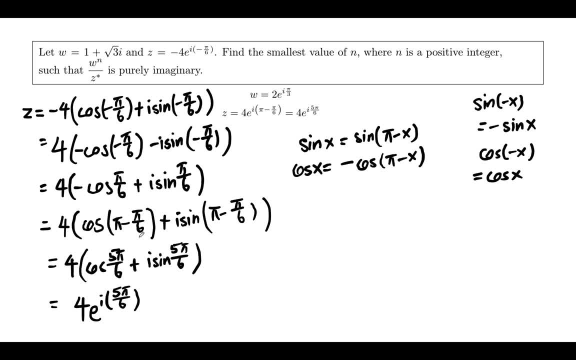 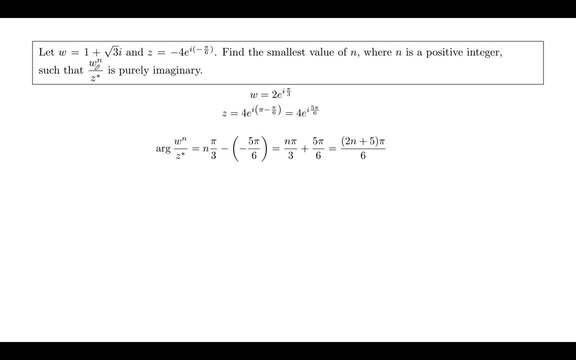 time to copy this down if you need to remember how, how we can do this. all right, so after doing that, we now try and find the argument of what they want: w to the n over the conjugate of z, because we know that for a complex number to be purely 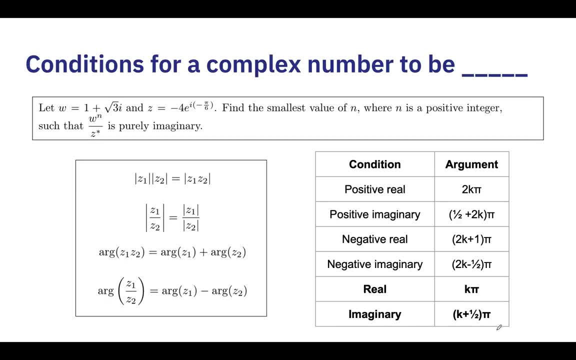 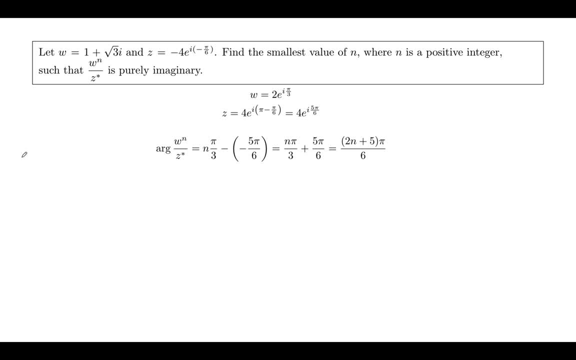 imaginary. we have to look at its argument. argument must be k plus half times pi. so when we find the argument, we can proceed to use some of the properties we know about argument and equate it to the difference between the argument of the numerator and the denominator right. so argument of w to the n is simply the 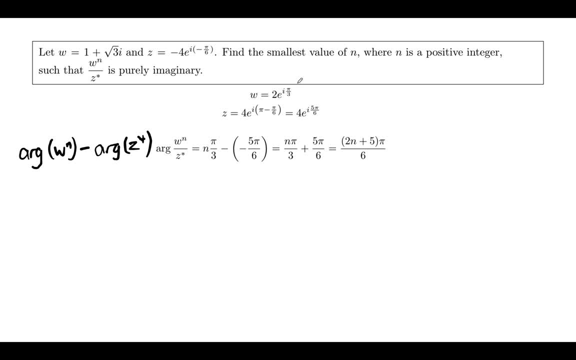 n multiplied by the argument of w, because if we raise this to the power of n, we are essentially multiplying this exponent by n. okay, and the argument of the conjugate of z is simply equals to minus, or the negative of the argument of z. right, so it's equals to minus 5, pi over 6, and if we simplify it, we get 2n plus 5. 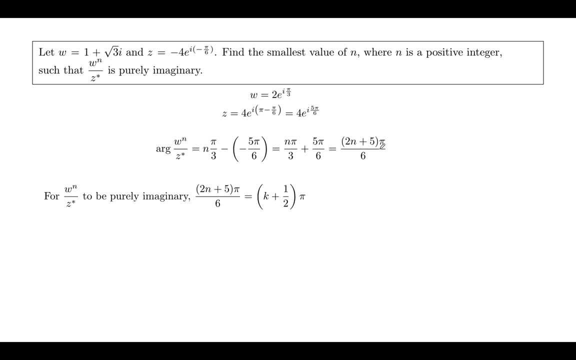 over 6 times pi. and we know that for the complex number to be purely imaginary, we get 2n plus 5 over 6 times pi. so we get this: 2n plus 5 over 6 times pi must be equals to k plus half times pi. so if we do some simplifications we'll find that the 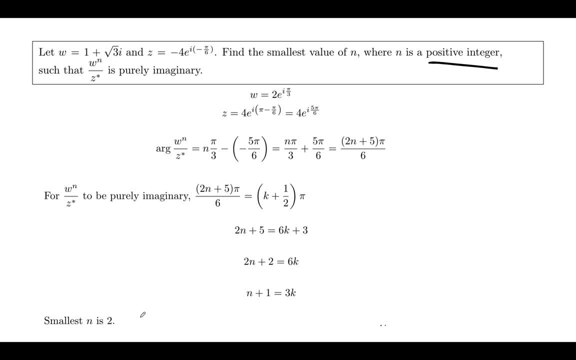 smallest n, where n is a positive integer, is, equals to 2, because the condition boils down to n plus 1 being a multiple of 3. so 2 plus 1 is n is 2. is the definitely the first positive integer that satisfies this condition. all right, so there's a rough guide on how we approach this type of. 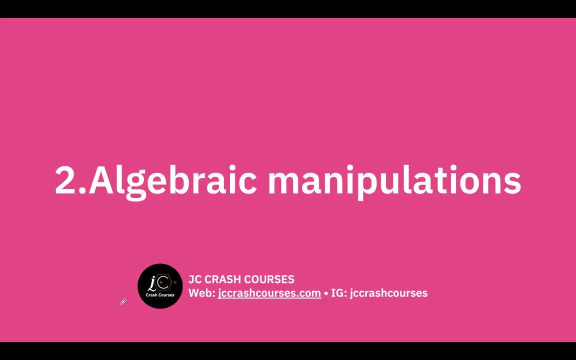 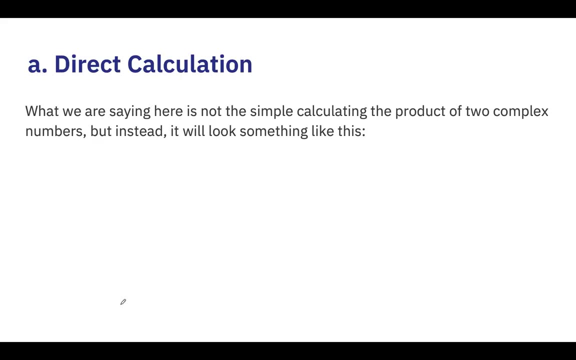 equation of questions. So next we're going to jump right into the topic of algebraic manipulations. So the first kind of question will be on direct calculation. So it's not a simple calculating of the product of two complex numbers, but instead it might look something like this: Okay, the question. 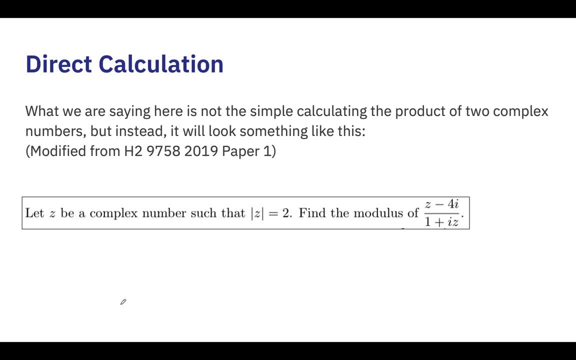 says: let z be a complex number such that the modulus of z equals to 2.. Find the modulus of z minus 4i divided by 1 plus iz. So pause this video. take a while to try this question. It's actually modified from the A-level paper, H2 mathematics paper 1 last year and I think it. 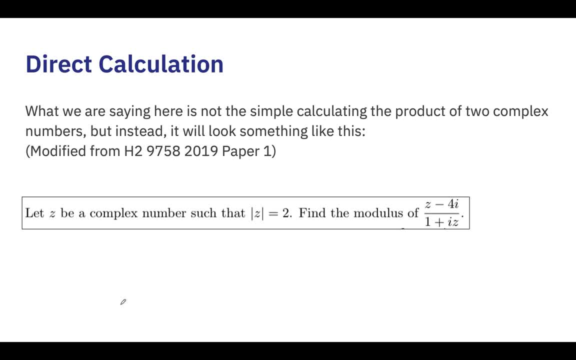 was one of the hardest questions in the paper, and I myself remember spending more than 20 minutes, or even half an hour on this question. Alright, so don't be afraid. don't be worried. if you can't solve it, just give it a shot and we'll review the solution after this. 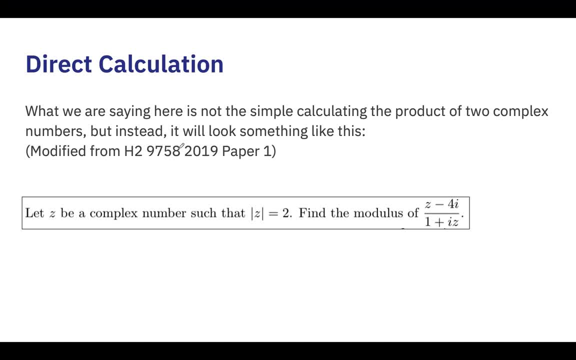 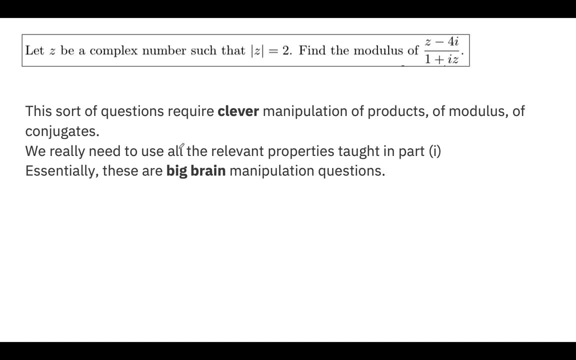 Alright, so we're going to look at this question now. So this sort of questions require clever manipulation of products, modulus and conjugates, So we really need to use all the relevant properties taught in part one. This is definitely on the harder end of the spectrum of complex. 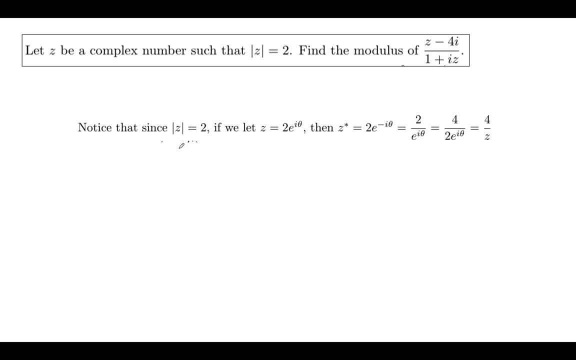 number questions. So we first notice that since the modulus of z is equal to 2, we can simply let z equals the 2ei to the theta and we get the conjugate of z to be 4 over z. And then we can take out the factor z from the numerator and with this 4 over z term over here. 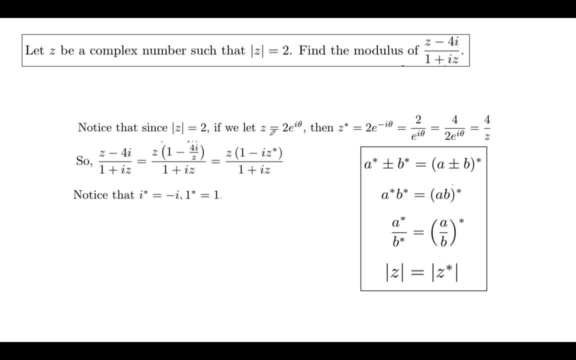 we can replace it with z conjugate And then we continue to use some properties and notice a few more things and we realize it will reduce very nicely to the modulus of z, which is equals to 2. So you can pause the video for a while. 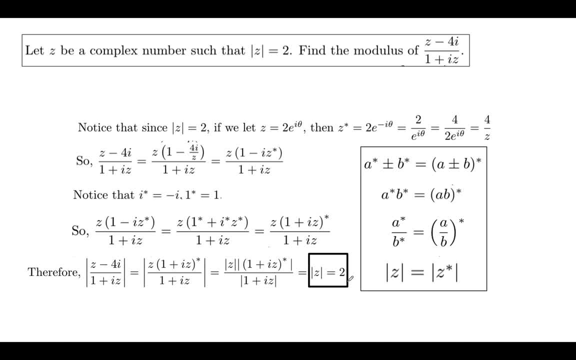 And take a look at all these steps and try and get how each step leads to the next. But, right, we see all these, notice, notice. and what if I can't really notice all these? it's very it's a lot to ask for, right, it's uh, it's not intuitive and in a stressful timed environment. 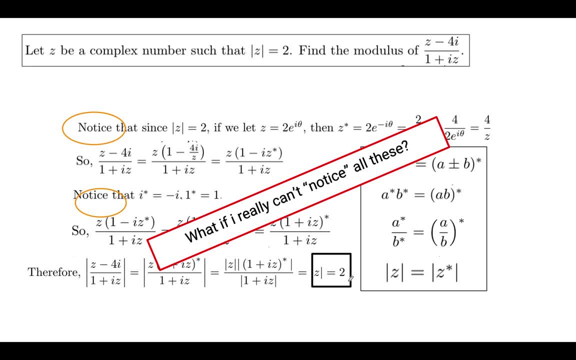 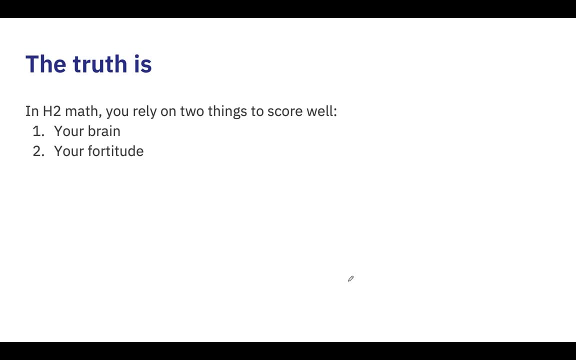 in an exam setting, it's very, very difficult to come up with all these uh from nowhere. So in h2 math you rely on two things to score well: either your brain or your fortitude. If one isn't working well, use the other. So if you can't seem to think of the very inspirational and motivated 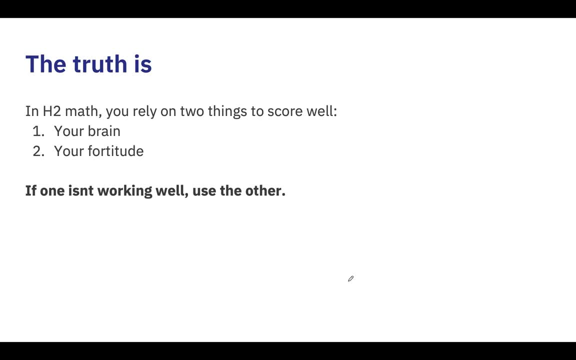 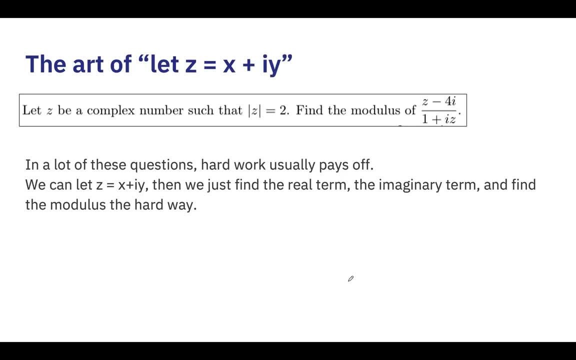 uh solution usually: uh, some kind of brute force or persevering long enough at a method known to definitely work will turn out well and give you the correct answer. Okay, so, as I said earlier, in a lot of these questions, hard work usually pays off. So what we're going to do is we can let z equal to 2.. 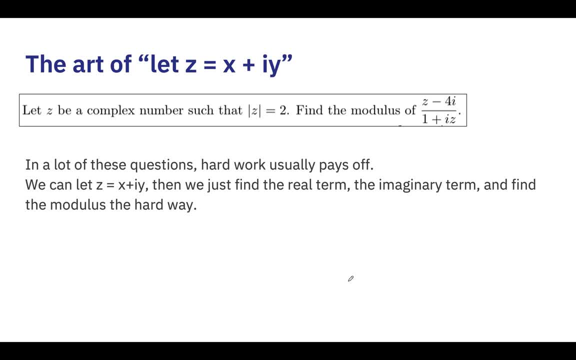 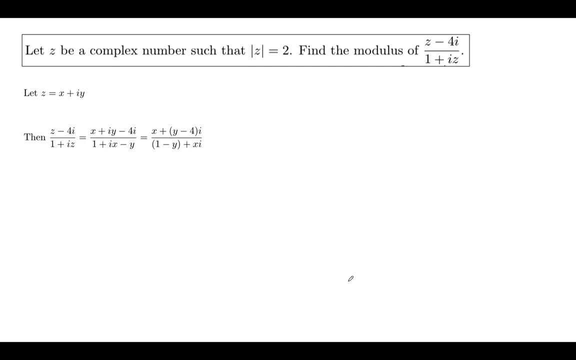 z equals to x plus i, y. this is a rectangular form of complex numbers. then after we do that, we simplify, we find the real term, the imaginary term, and then we find modulus the hard way, using the pythagoras theorem formula. Okay, so when we let z equals x plus i y, we substitute it in into both z. 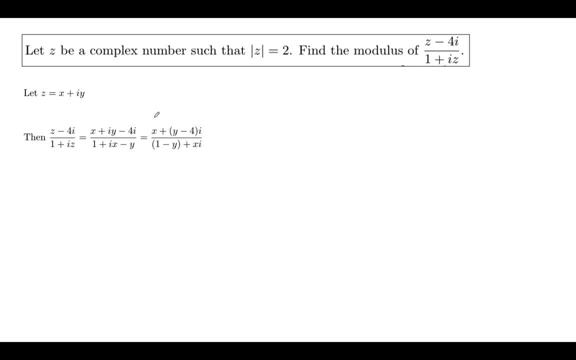 terms in the numerator and the denominator. Okay, and then we try and write it neatly in terms of its rectangular form, both on top and on the bottom. Okay, and then the next thing we do is we rationalize the denominator by multiplying it by its conjugate, which is 1 minus y minus xi, and we have to multiply the same to the top as well. 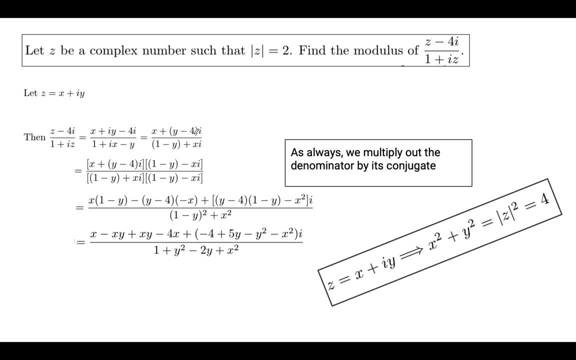 And then we just have to do some algebraic expansion and we will get this form over here: minus 3x plus minus 8 plus 5y times i over 5 minus 2y Right. and another thing I want you to notice is: 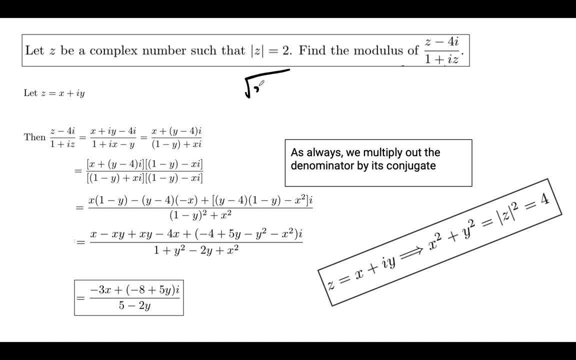 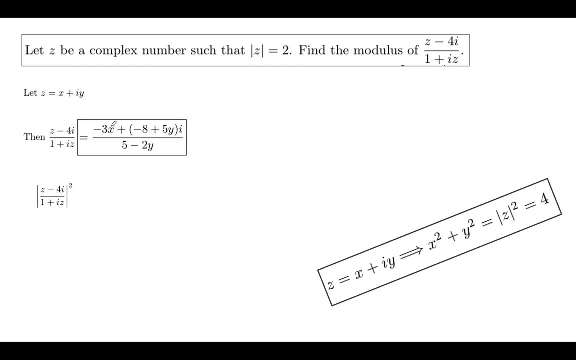 that when we write the formula for the modulus of x plus i, y, right, the formula for the modulus is simply square root of x square plus y squared, and this is equals to 2.. So x plus x squared plus y squared actually equals 4.. Okay, so, remembering this, we have our form over here, right, our form. 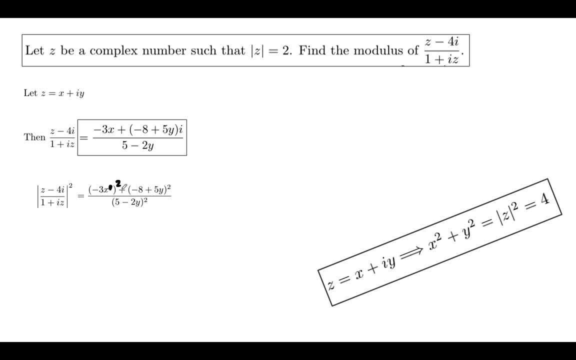 and then now, what we want to do is we want to find the modulus squared. So, in order to do sorry, the square is supposed to be outside. In order to do this, we can realize that this is actually x over 5 minus 2y plus minus 8, plus 5y over 5 minus 2y, i Right, so this is actually a complex. 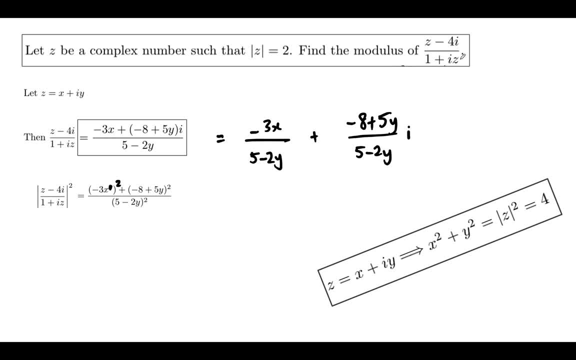 number in a rectangular form because we were able to change the denominator to a real number by rationalizing the denominator. So if you want to find the modulus of this squared, it's simply taking this term: squared plus the coefficient of i squared Right, which is equals to this, and if we simplify it and use x squared plus y squared, equals to 4. 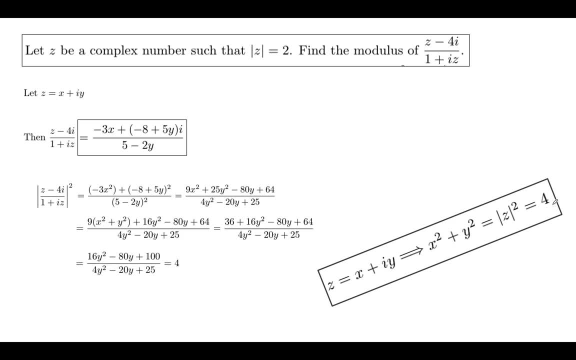 we will be able to get it very nicely reduced to be exactly equals to 4. And therefore the modulus of z minus 4i over 1 plus i z is equals to 2. And we have to reject minus 2, of course, because we 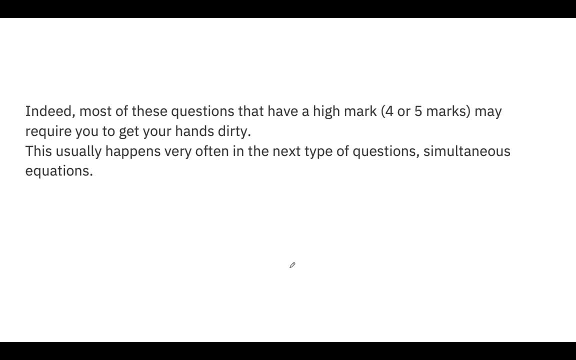 know that modulus must be non-negative, Right? so, as we can see, most of these questions that have a non-negative answer will require you to get your hands dirty, especially if you can't think of the most elegant solution, Right? so this usually happens, very often in the next type of questions. 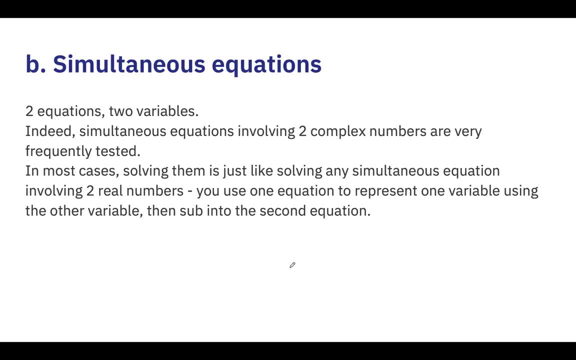 on simultaneous equations. So the simultaneous equations that are tested in a complex numbers topic would contain two equations and two variables. So these are very frequently tested and in most cases solving them is just like solving any simultaneous equation involving two real numbers. You use one equation to represent one variable using the other variable, then you substitute it. 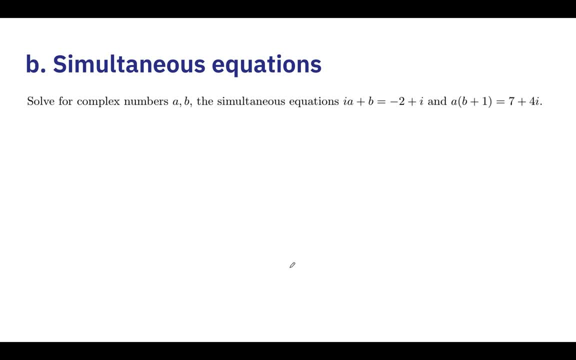 into the second equation. So a basic example would look like like like. so for solve for complex numbers, a, b, the simultaneous equations i, a plus b equals to minus 2 plus i, and a multiplied by b plus 1 equals to 7 plus 4i. Okay, so keep in mind a and b. here are complex numbers. 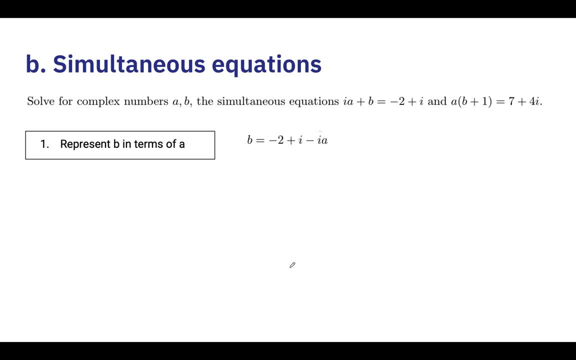 First, we want to represent b in terms of a, and we can do this very easily using the first, the first equation over here, right this one, and once we do this we can substitute it in into equation two, and then we do some simplifications. Now we have an equation in terms of a only, 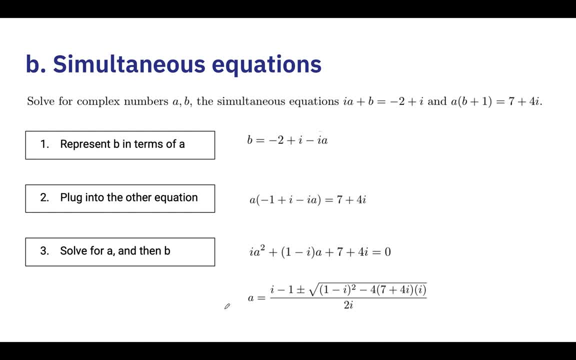 so we can actually use the quadratic formula. Do remember: the quadratic formula still works. even though your coefficients are not real right, it still works. So if we key in to the quadratic formula, or if you use your gc rather, you'll get a equals to 2 plus 3i or minus 1. 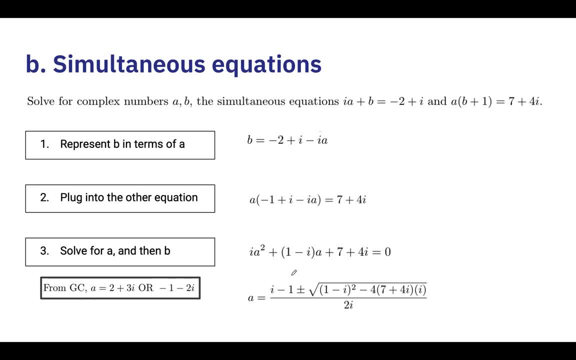 minus 2i. Okay, as far as i remember, we can't use the scientific calculator to key in complex coefficients, so you have to use your gc's equation solver. Okay, so after we get our values for a, we can then find the corresponding values for b, and we will then have solved our simultaneous. 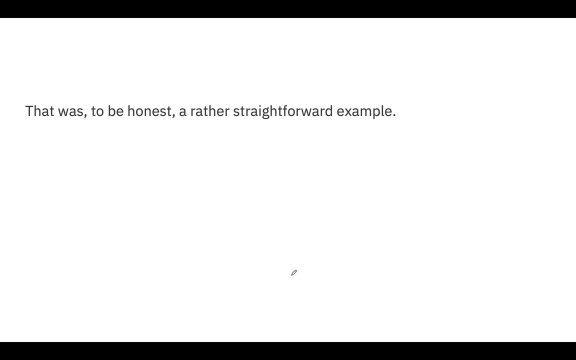 equations Right. so, as i said earlier, this is a rather straightforward example, but if you want to test it, you can use some other equations. but i'm just going to show you a simple example. A complex number can have a conjugate and modulus, so they may like to test that. 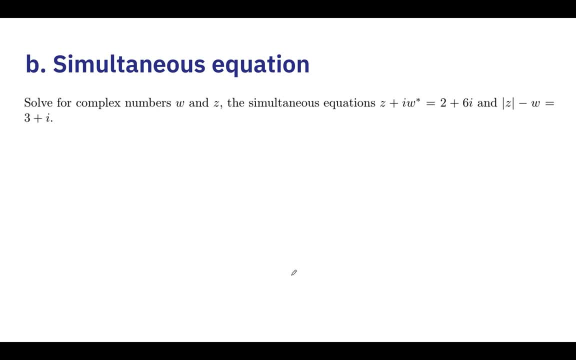 in these linear equations as well the simultaneous equations, right. so here we have another, harder question that asks us to solve for complex numbers, w and z. The simultaneous equations. z plus i multiplied by the conjugate of w equals to 2 plus 6i equals to 3 plus i. so substitution looks like an absolute mess here because we have conjugates and 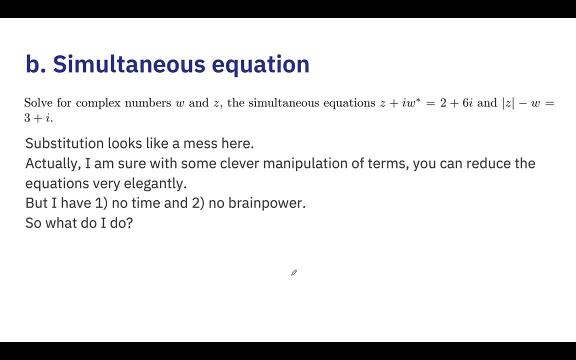 we have modulus. there's a lot of things to take care of, right, and this question can probably be done using, you know, an elegant solution, the kind of solution that you expect in the answer key, right. but here, if we have no time and no brain power to come up with these kind of things, 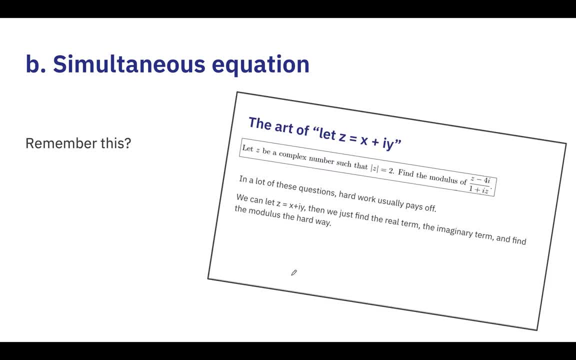 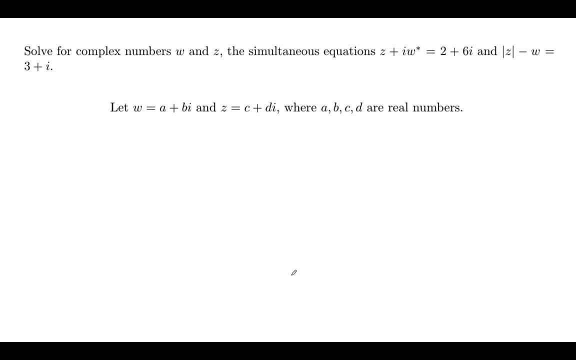 what are we going to do? we have to rely on our fortitude, and we can do the so-called brute substitution by replacing z with x plus iy. it's rectangular form, right? Halberd usually pays off with this kind of substitutions, so that's exactly what we're going to do. we're going. 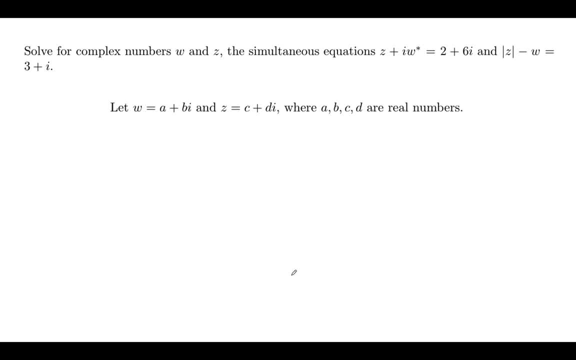 to replace w with a plus bi and z with c plus di, and we're going to bash this out, okay. so what we're going to do here is we are going to substitute in- uh, these two rectangular forms into our equations. here we start with the first equation right: z equals to c plus d, i, c plus d, i plus i, multiplied by. 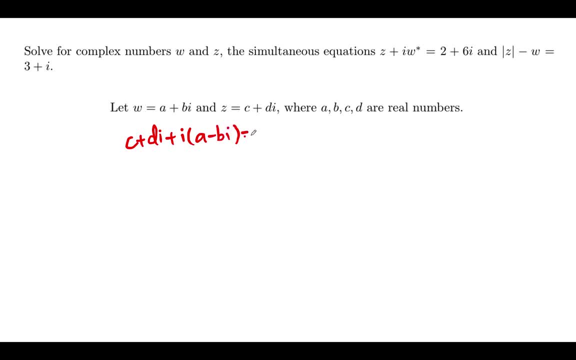 the conjugate of w equals to 2 plus 6 i. and if we do some simplification here, we get c plus b plus a plus d i equals to 2 plus 6 i. so, comparing coefficients, we get b plus c equals to 2. 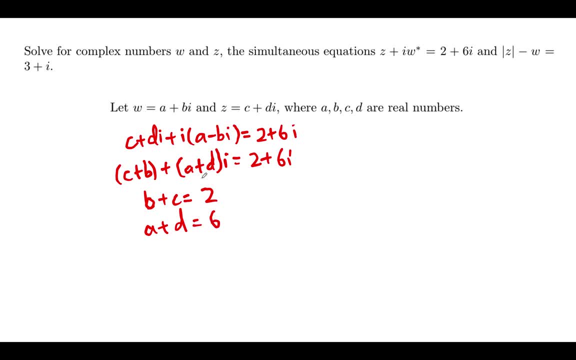 and a plus d equals to 6.. right now we look at the second equation. mod of z minus w equals to 3 plus i. so the mod of z is equals to square root of c squared plus d. squared minus a minus b, i equals to 3 plus i. right, so if we do some simple reshuffling we get a plus 3 plus b plus 1 all. 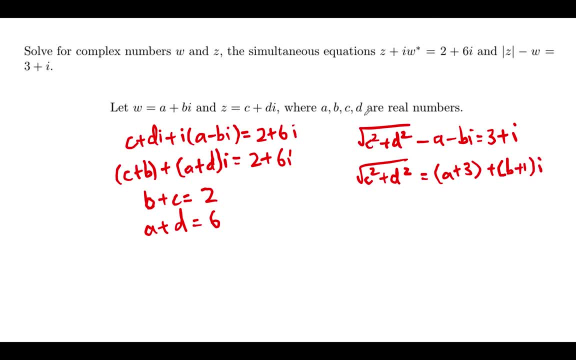 right now. we know that c and d are binaries, so we can't do the headlights and delta. well, we know that c and d are binaries, so we can't do the Orchestralster's, so we can't both real numbers as defined. So this square root here has to be a real number as well, because we 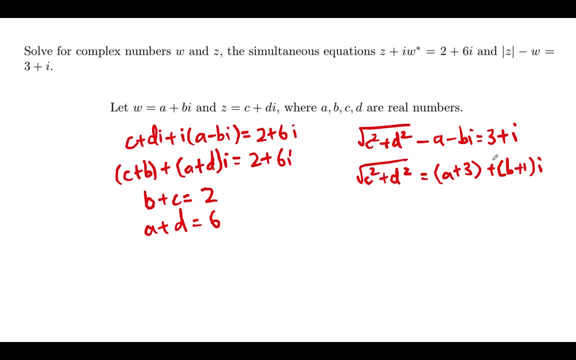 are adding the squares of two real numbers, which must be non-negative, So this means that it cannot contain an imaginary part, or rather, this term is equal to 0.. So, since b plus 1 is equal to 0, b is equal to minus 1, and using this equation over here, we get c equals to 3.. And now what we are? 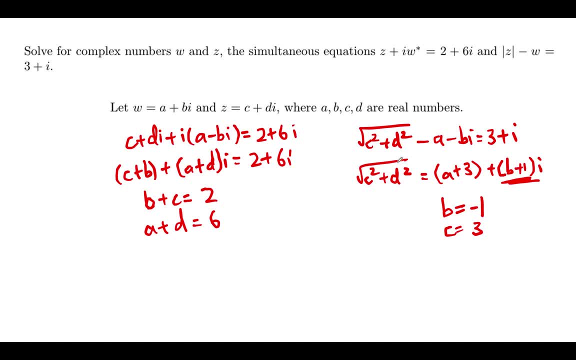 going to do is substitute in these values c equals to 3 into this equation. So we get 9 plus d. squared equals to a plus 3, and a is equal to 6 minus d, So it becomes 9 minus d and now we have an equation. 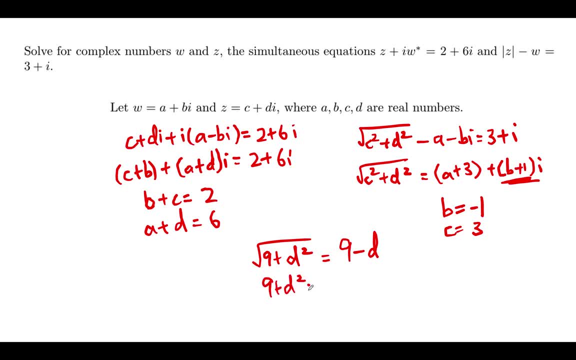 in one variable. If we square both sides, 9 plus d squared equals to 81 minus 18d plus d squared. Okay, so the d squared cancels out. 18d is equal to 7.. 2 and d is equal to 4.. And if we substitute back in here, we get a equals to 2.. So w is equal to 2 plus 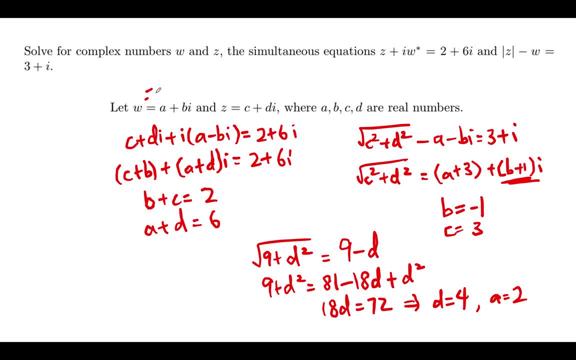 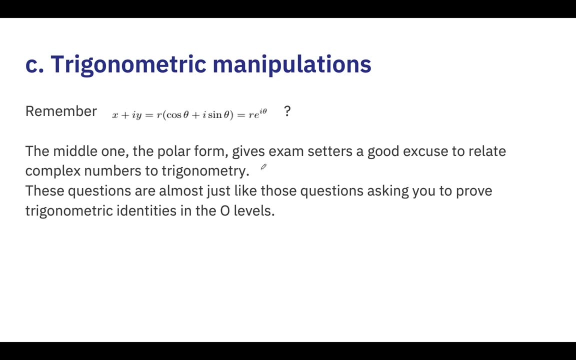 b, i, which is minus 1.. So it's equal to 2 minus i, and z here will be equal to 3 plus 4i. Simple as that. Yeah, so do you all remember this trigonometry, this identity that we have? 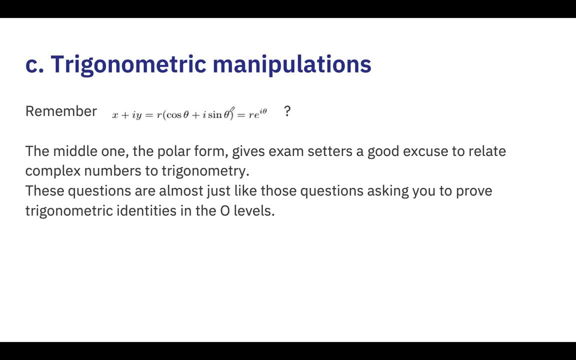 already. So we have this identity here and we have this identity here and we have this identity here. So we have this identity here and we have this identity here. So we have this identity here And we have this identity over here, converting between rectangular form, polar form and. 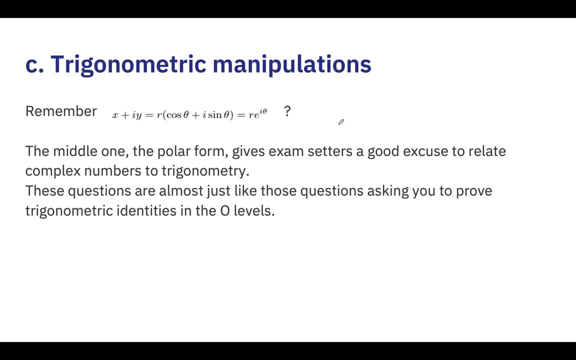 exponential form, The middle one, the polar form, gives exam setters a very good excuse to relate complex numbers to trigonometry. So these questions are almost exactly like those questions asking you to prove trigonometric identities in the O Levels and, honestly, they can be quite Siena, because they are testing you on both complex numbers. 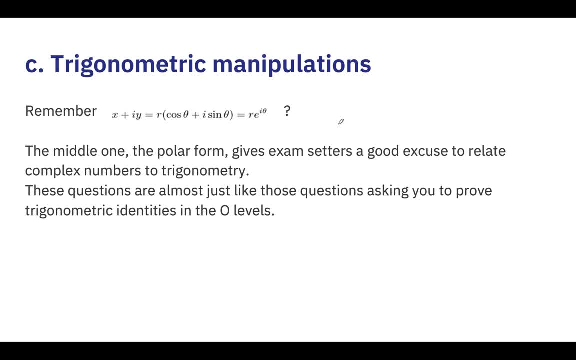 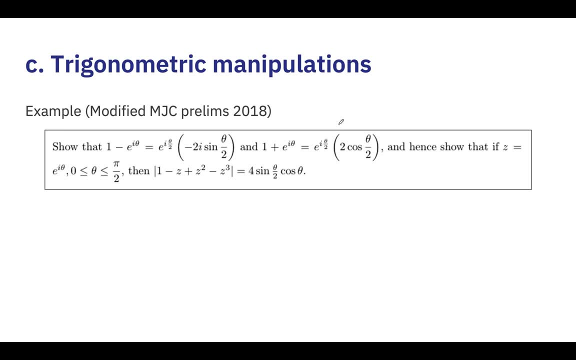 and trigonometric identities and manipulations, But all you need to do is to push through and it and press on Alright. so we have an example for you to try over here. It's modified from MJC prelims 2018.. It's a two-part question. The first part asks: 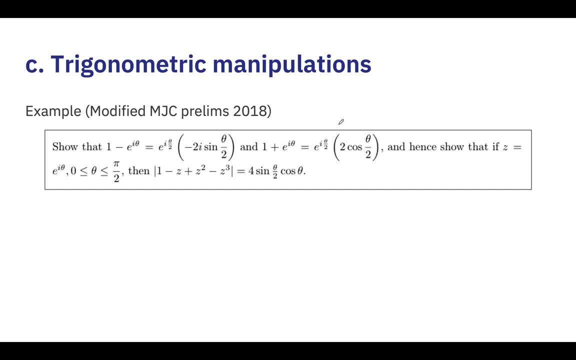 you to show some properties, some identities that contain both exponential form of complex numbers and sine. And then the second part of the question is a hands part that asks you to prove this identity, that absolute, the modulus of 1 minus z, plus z square minus z cubed, equals to some kind of trigonometric. 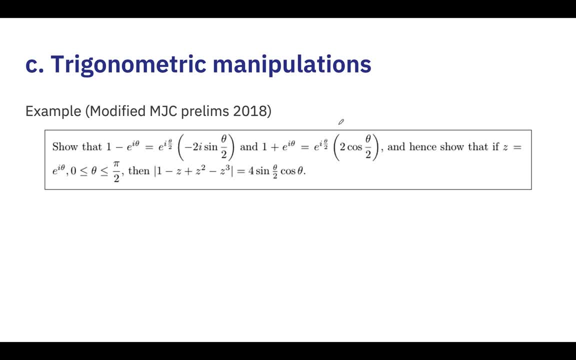 identity. So do pause the video, give this question a short, give it your best shot, in fact, and after this we'll go to the solution. Alright, so we're going to be starting with the first part of the question first. So it asks us to show that 1. 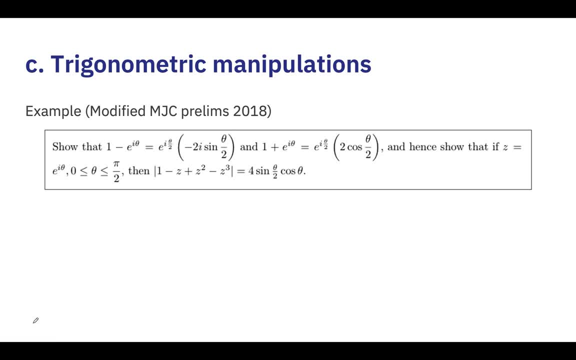 minus E to the i theta is equal to this expression shown over here And, as you can see, this expression shown over here has an e to the i theta over 2 term factored out. so we're going to try and do that right if we. 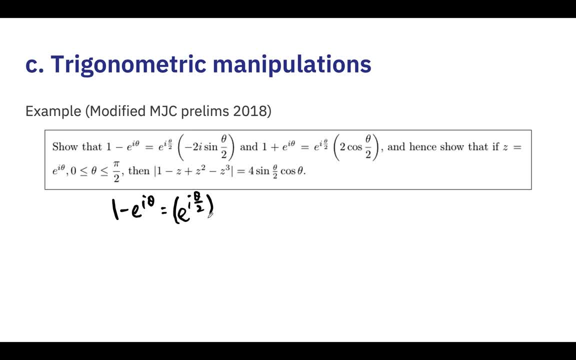 factor this out, we'll be left with e i minus theta over 2, minus e i theta over 2, right, and then we can write each of these terms here in their polar form, because you want to get like in terms of cosine and sine and hope you know the cosine terms. cancel out, so be cosine minus theta over 2. 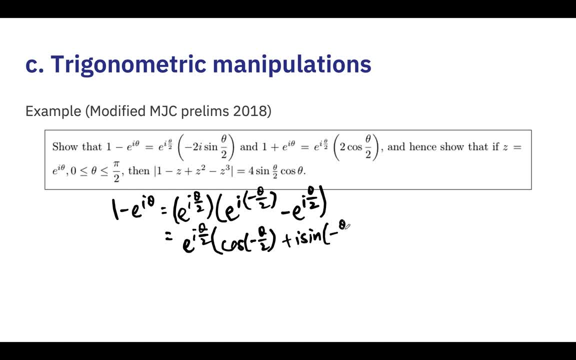 plus i sine minus theta over 2, minus cosine theta over 2. minus i sine theta over 2. and the next thing we have to do is to convert each of these angles in here into their positive versions so that we can do the cancellation. so we recall that cosine of minus x is equals to cosine of x. 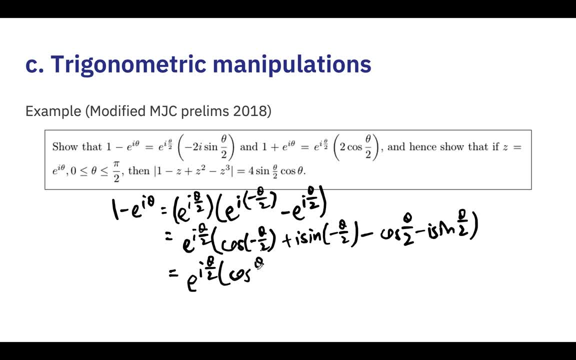 so we can do the cancellation, and then we have to convert each of these right, so we can simply remove the negative sign, but for sine we have to bring out the negative sign, so it becomes: minus i sine theta over 2. minus cosine theta over 2. minus i sine theta over 2. 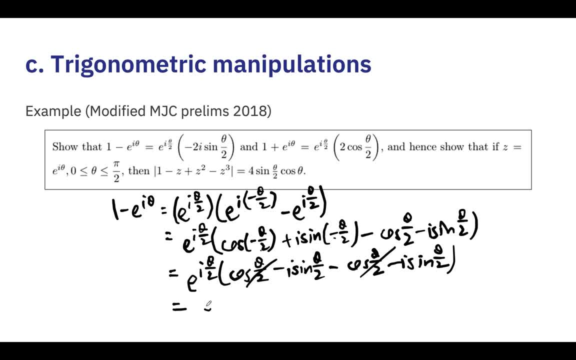 so now we can cancel the cosine terms out and we will get the desired result. okay, so for the other case, it's almost exactly the same. so do try it out. and essentially what you're doing is you're going to get the negative sign and then you're going to get the cosine. 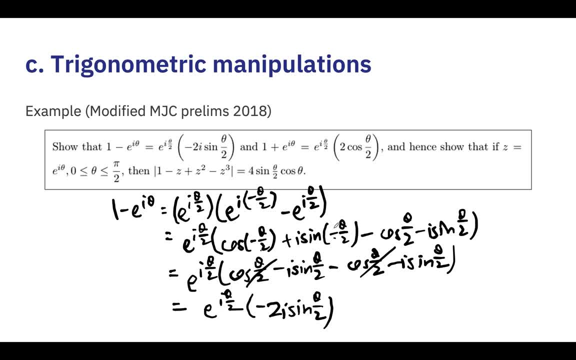 terms out. so what you're doing is you're replacing this with a addition sign, so these all become pluses, and instead of the cosine terms cancelling out, now your i sine terms cancel out, leaving 2 cosine theta over 2. okay, so now we're gonna try the second part. 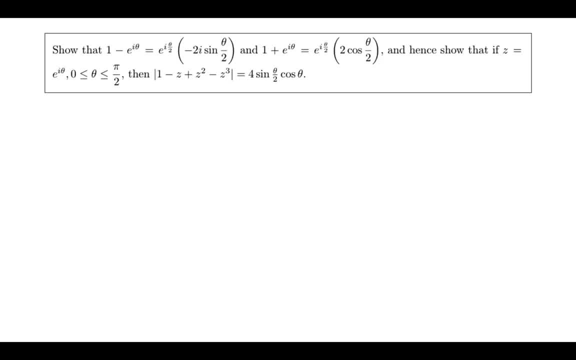 all right. so next we have to solve the second part of this question. right, and the word hence here gives us a very good starting point, right? this word hence here tells us that the cosine terms that we have to try and use what we derived in the first part of the question in order to maybe try. 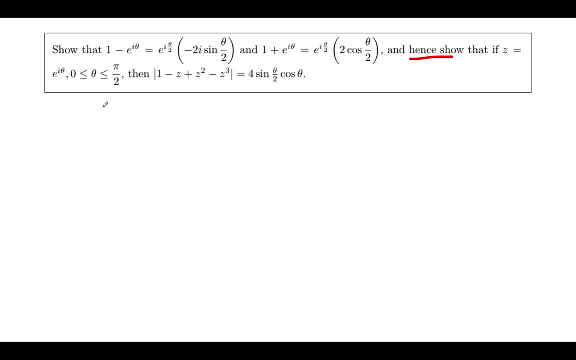 and solve this very weird identity. okay, so the first thing we're going to do is rewrite this thing inside the modulus. 1 minus z plus z squared minus z cubed is equals to: we can factor out the z squared for the remaining two terms and it will look something like this: and then, if you recall, we: 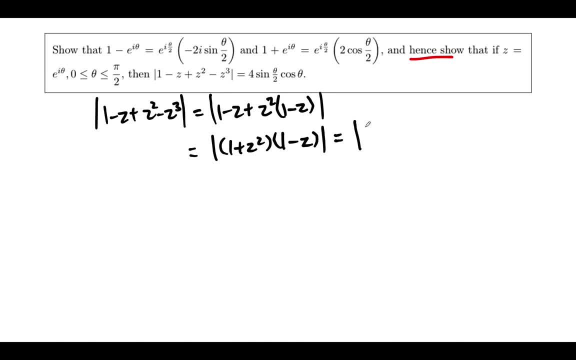 can actually separate the products, so we will get something like this all right from our properties to do with modulus. okay, so we know that we actually have this 1 minus z here already, so what we need to take care of is the 1 plus z squared. okay, so there's something we 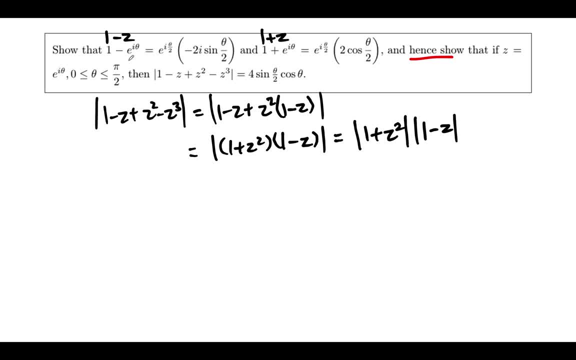 can do that looks very attractive, which is to actually multiply these two things over here. okay, why is this a very attractive thing to do? is that because multiplying these two will give us 1 minus z squared, which is, you know, kind of close to what we need, and then maybe we can try and find z later. 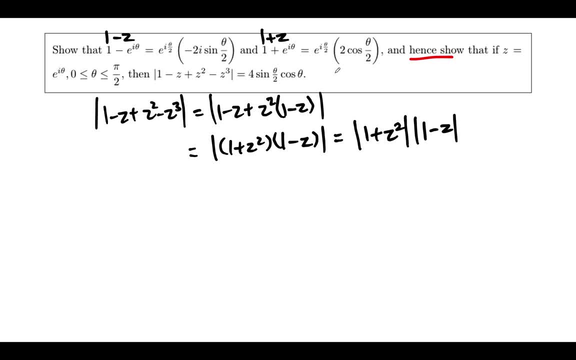 in terms of these and find 2z squared and then add it. okay, so that's the first thing we're going to try, right? so 1 minus z squared will be equals to the product of these two. these two will combine to become ei, theta, and then we multiply these two brackets. we get minus 4. 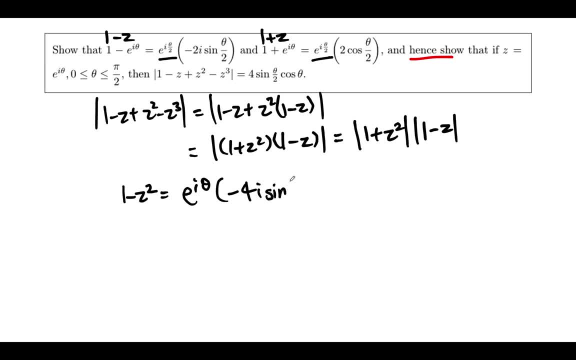 i sine theta over 2, cosine theta over 2 right. and then now we have to find 2z squared. so next we are going to take this and subtract it with this. so 1 plus z minus 1 minus z will give us ei theta over 2. 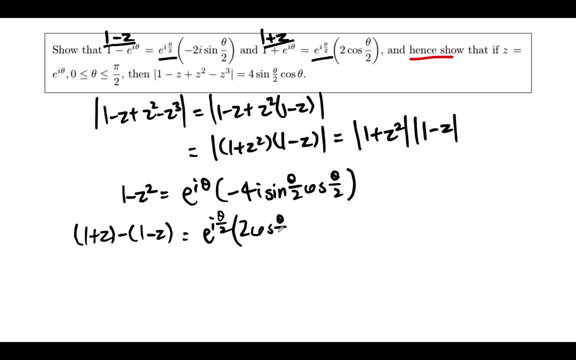 2 cosine theta over 2 minus minus 2i sine theta over 2, so it becomes plus, right. so this is actually equals to 2z and is equals to 2 ei theta over 2 cosine theta over 2 plus i sine theta over 2. 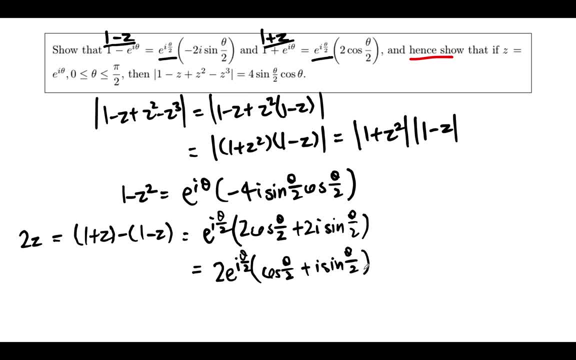 right, so we can just cancel out the 2 and we'll get z equals to e, to the power of i theta over 2 times cosine theta over 2, plus i sine theta over 2. and next we want to square this, because when we square it then we can multiply it by 2 and add it to this. 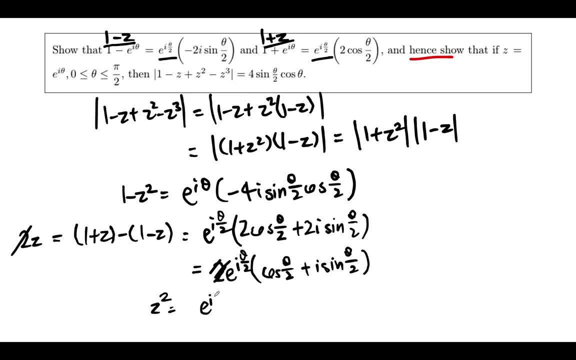 so when we square it, we get ei theta, then the inside will become cosine squared theta over 2 minus sine squared theta over 2 plus 2i. cosine theta over 2 sine theta over 2 right. and then remember, we want to find 2z squared, not just z squared, because we 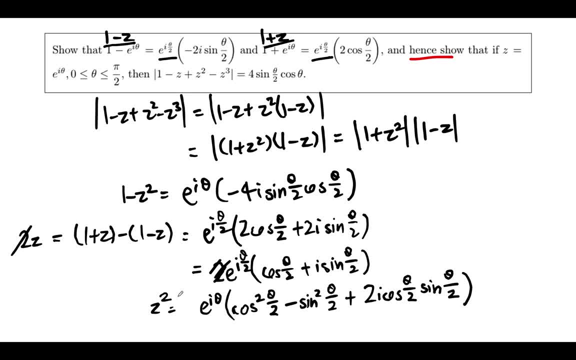 need to add 2z squared to this in order to get 1 plus z squared right. so if we multiply this by 2, there will be a 2 that comes out here, an extra 2 here and this will become 4. okay, so this might all look very complicated, but we realize that. 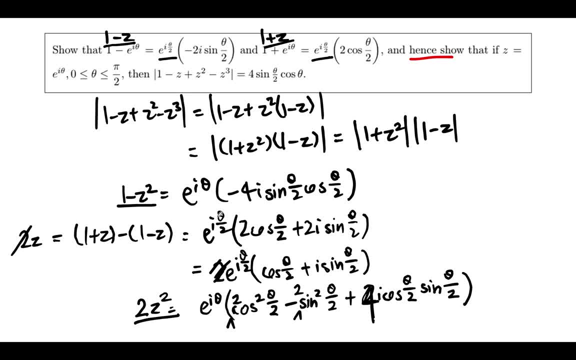 when we add this and this term together, we have the same uh, same factor, right ei theta, and this 4i sine theta over 2, cosine theta over 2 will cancel out with this one over here, which makes it very beautiful, and all we are left with is: 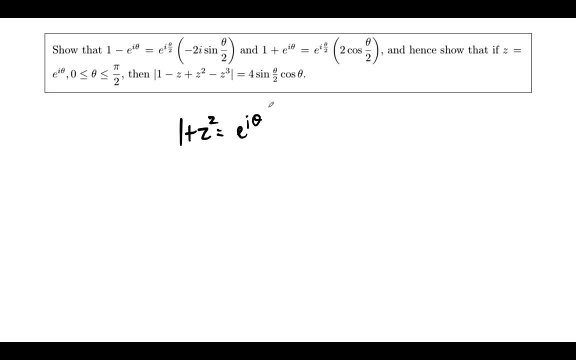 1 plus z squared equals to ei theta. we just have to look at these two terms over here, right, because the other two will cancel out. so we get 2 cosine squared theta over 2, minus 2 sine squared theta over 2, and we can factor out the 2. 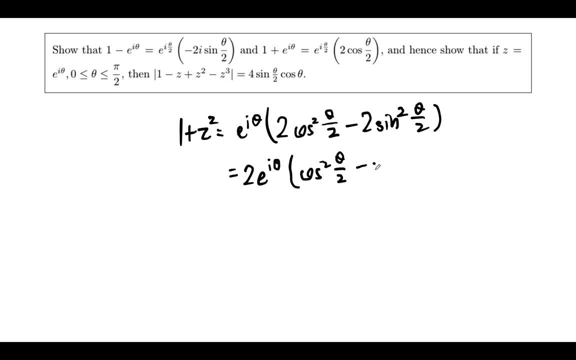 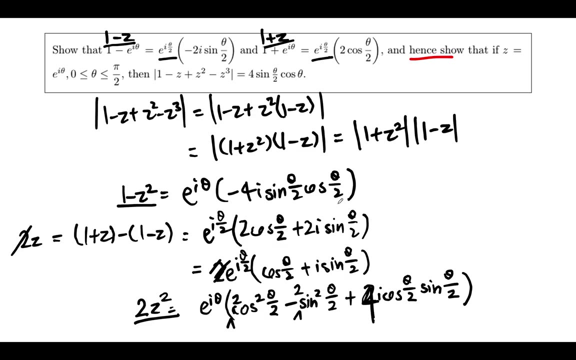 this becomes cosine squared theta over 2, minus sine squared theta over 2, and if we know our double angle formula, this thing right here is actually equals to a very nice result: cosine theta. that's it, right, okay? so if we realize, what are you looking for here? they're looking for: 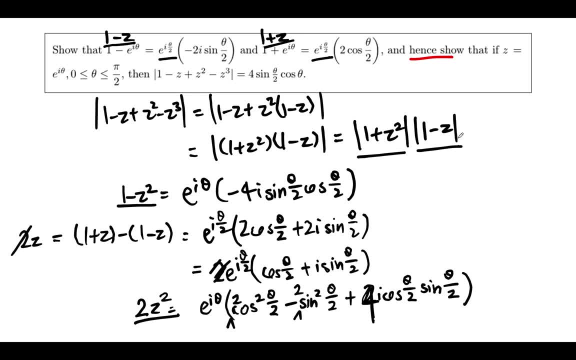 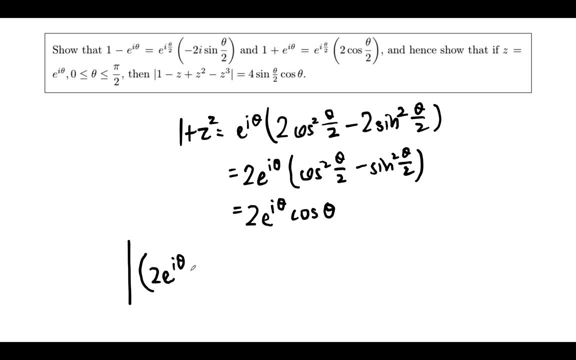 the modulus of this multiplied by the modulus of this. okay, so actually there isn't really a need to separate it out, but it might help you see a little easier. so if we multiply inside it becomes the modulus of 2, ei, theta, cosine theta, and the other term would be 1 minus z, which is this thing over here. 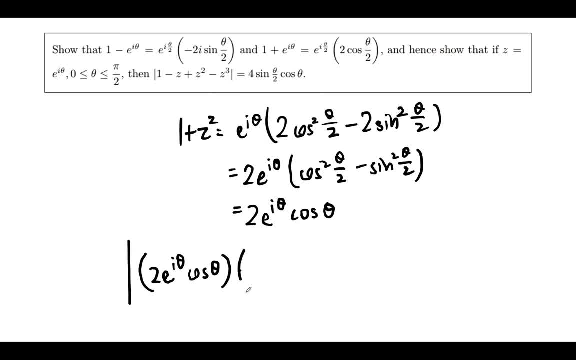 so we're just going to copy it: e i theta over 2 minus 2. i sine theta over 2. okay, and now we want to try and simplify the thing inside a little bit. becomes, becomes minus 4, minus 4. e to the i: 3 theta over 2. 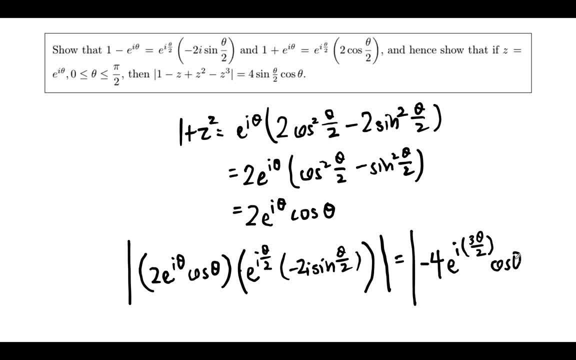 cosine theta sine theta over 2 right. so, as you can probably see, the this thing is starting to really look like what we want, right, and we're actually done, because this is the complex number over here, right. e to the power of i: 3 theta over. 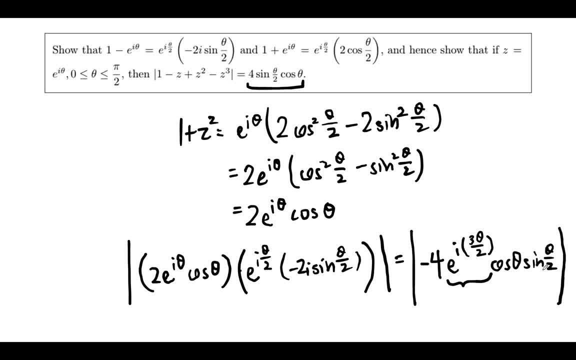 2. this is the exponential form, this is the complex number, so everything else must be part of the modulus. so the modulus of this is simply the modulus of everything, excluding the complex number, which is equal to four cosine, theta, sine, theta over two. and we've shown the identity. 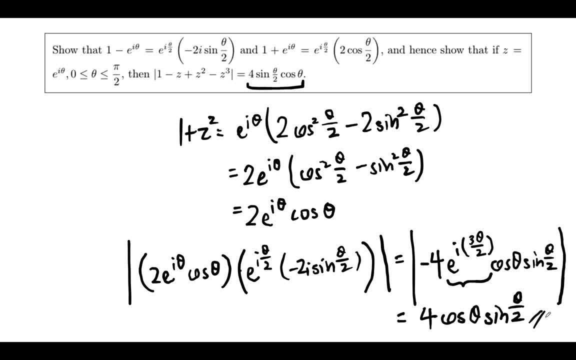 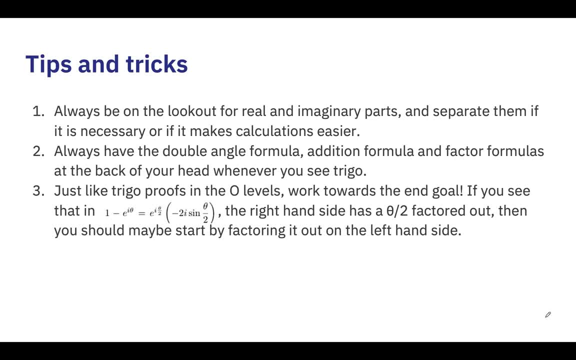 okay. so this is one of the hardest possible questions they can ever test to do with trigonometry, so don't worry if you can't solve it right. so some tips and tricks for these types of questions: always be on the lookout for real and imaginary parts and separate them if it is. 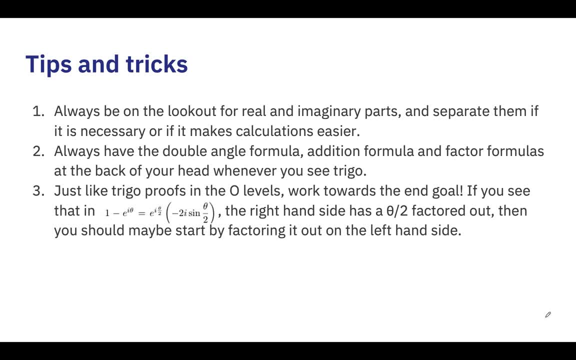 necessary or if it makes calculations easier. right and always know the double angle formula, addition formula and factor formulas right at the back of your head, right whenever you see trigonometry and, just like trigger proofs in the o levels, try and work towards the end goal. so if you see that in this identity we had just now, the right hand side has a theta over two, 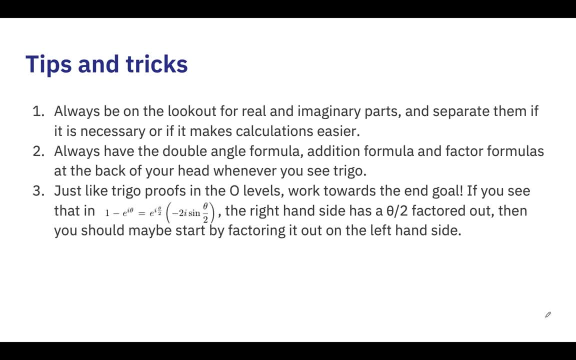 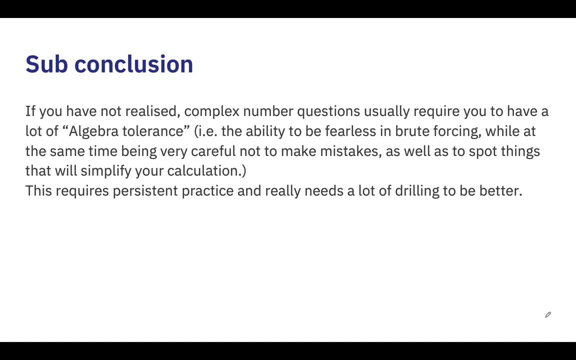 factored out, then we want to try and start by factoring it out on the left hand side. okay, so if you haven't yet realized yet, complex number questions usually require you to have a lot of tolerance for algebra, and which is basically the ability to be fearless in expanding out everything in brute forcing and, at the same time, being very 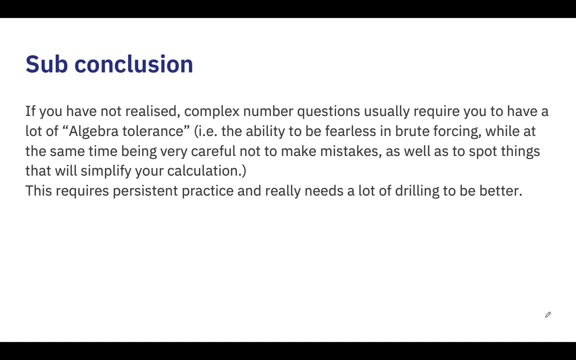 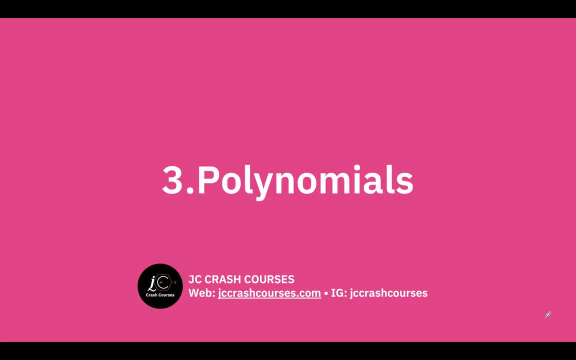 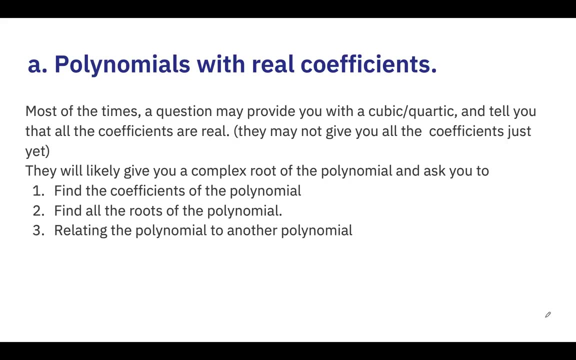 careful not to make mistakes as well as to spot things that will simplify your calculation, and this really requires a lot of persistent practice and a lot of drilling to get better right. so for the final chapter of this topic, we are going to look at polynomials. so the first aspect of this would be polynomials with real coefficients. 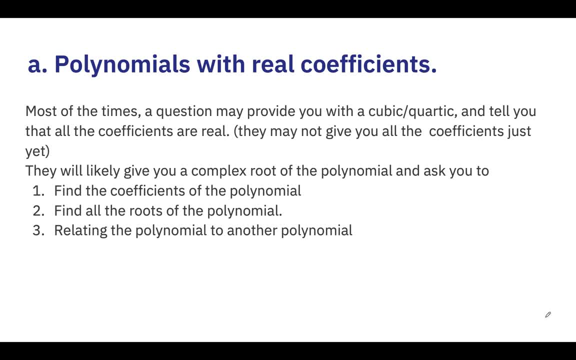 so most of the time, a question may provide you with a cubic or maybe even a quartic and tell you that all the coefficients are real, and they may not give you all the coefficients just yet. okay, so there are three kinds of things they can ask for. they will likely give you a complex root. 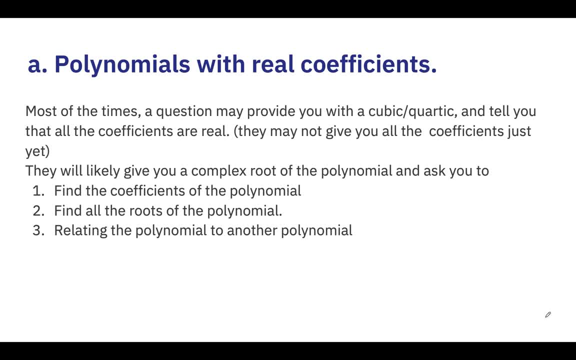 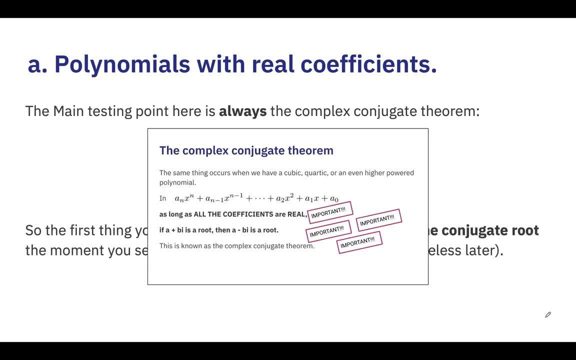 of the polynomial and ask you to: number one, find the coefficients of the polynomial. number two, find all the roots of the polynomial. and number three, relating the polynomial to another polynomial right. the main testing point for polynomials with real coefficients is always the complex conjugate theorem. okay, so the complex conjugate theorem states that uh. 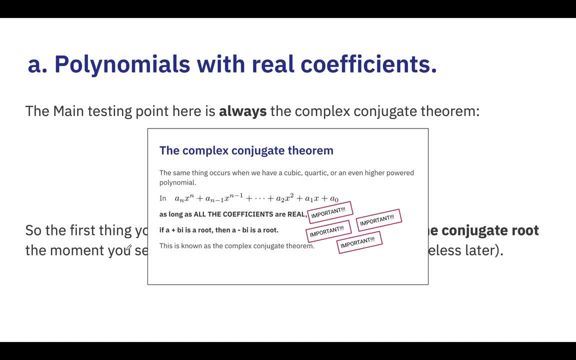 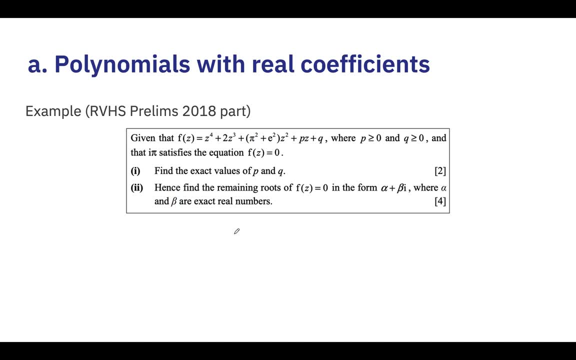 see, as long as all the coefficients are real, if a plus b i is a root, then a minus b i is a root. so we have an example over here. so pause this video, give it a shot and we're going to go through the solution after this. 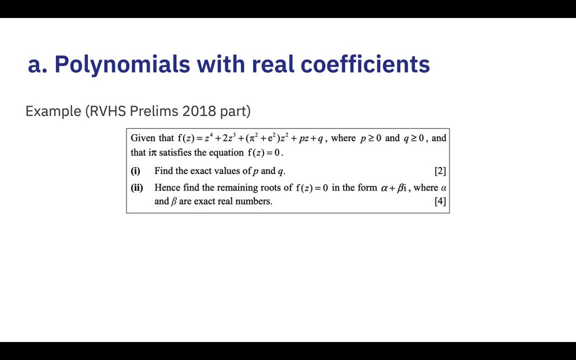 all right. so we're going to look at this question. given that uh f of z is equals to z, to the 4 plus 2 z cubed plus pi squared plus e, squared z squared plus p, z plus q, where p and q are both non-negative reals, and that uh i pi satisfies the equation f z equals to zero. so part one asks us to: 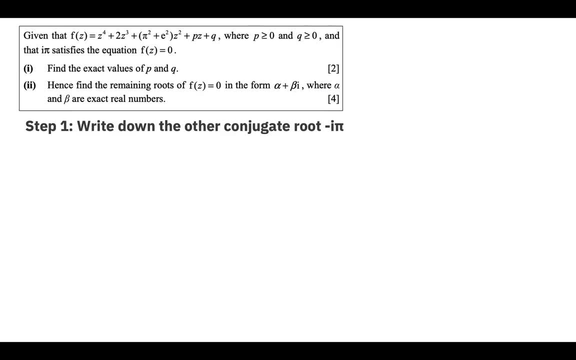 find the exact values of p and q. so first, since that, since i pi is a root uh, using the theorem, we know that the other uh, the conjugate of i pi, which is minus i pi, is also a root, right. so the trick here is to plug in the roots one by one, and after that you'll get simultaneous equations relating. 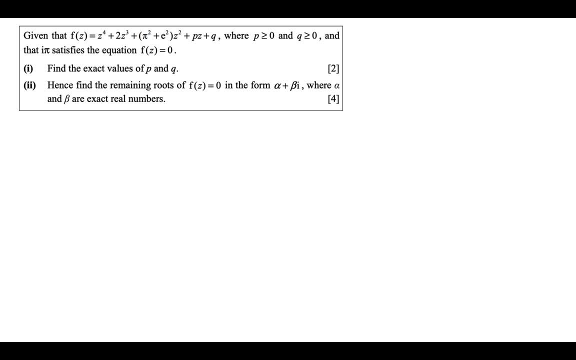 the coefficients that can be solved right. so now we're going to plug in uh. we're going to plug in uh i pi the minus i pi. so all right, so we know that. uh, sorry, we know minus i pi is a root, but maybe we can try plugging in i pi first. uh, when we plug in i pi, we get uh pi pi to the 4 plus 2 i pi. 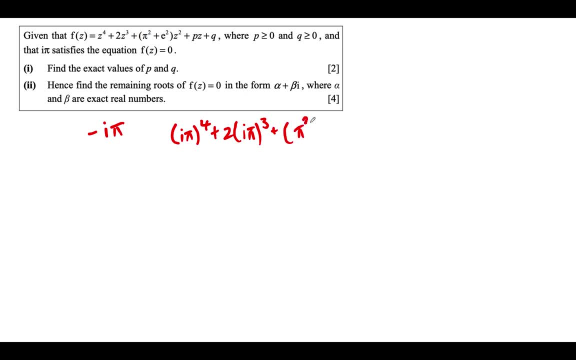 to the 3.. so we just write it out neatly: first right, and then we simplify this, so this becomes, this becomes our minus pi squared, so minus pi to the 4 minus right, and then we can cancel these two out, and then it becomes: uh, we group the imaginary terms together and the real terms together. 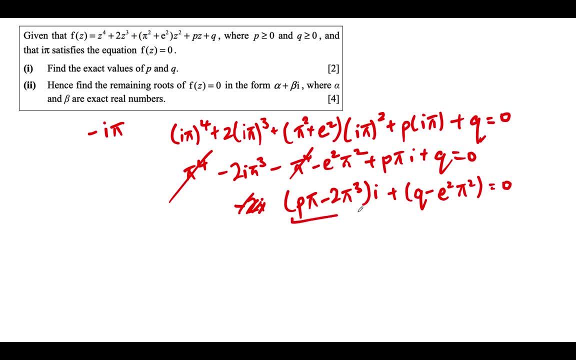 right, so this is equals to 0. we know that this is 0 and this is 0, so q is equal to e squared pi squared, and p is equal to 2 pi squared. right, so we've been able to find the exact values of p and q, hence find the remaining roots of f, zero, which is equal to 1 pi. 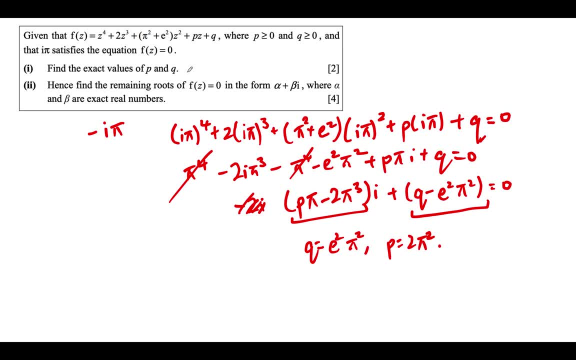 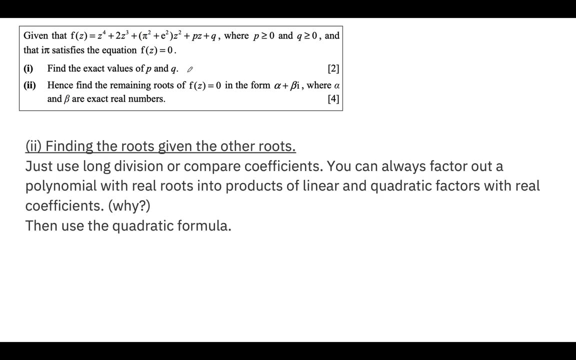 save for one second start from this stage, and we'll talk a little bit later about d z wedding fermin z equals 0 in terms, in the form of alpha plus beta i, where alpha and beta are exact, real numbers, right? so how are we going to approach this question, right? uh, what we're going to do is 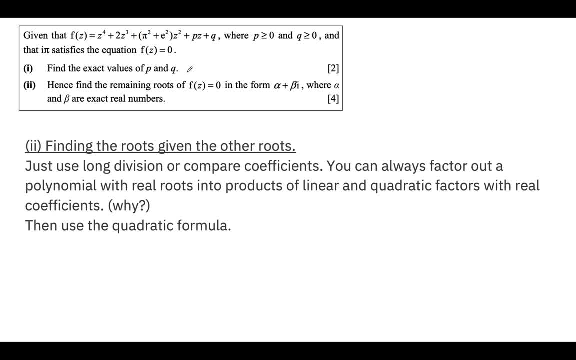 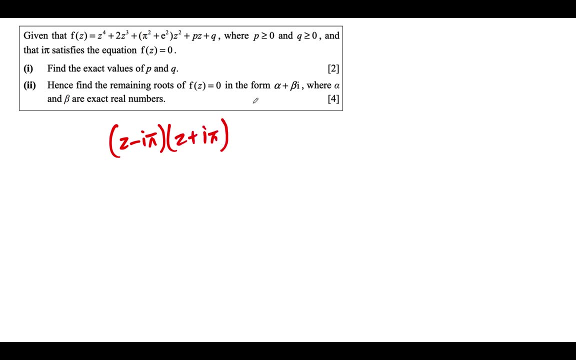 we're going to sub in both i pi and minus i pi, and then we try and factor out a polynomial that we can solve with quadratic formula. okay, so we know that one of the factors to this thing is z minus i pi, since i pi is a root and z plus i pi is also a root right, and this is equals to z. 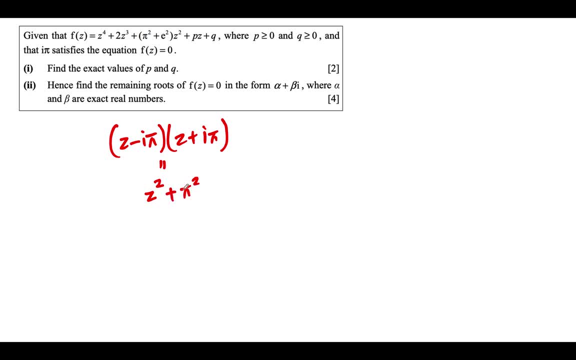 squared, uh, plus pi squared. so really our remaining quadratic here is just z squared plus az. and then our q here is e squared, pi squared. so our constant term comes from here: e squared, right. and really all we have to do now is to compare quadratics, coefficients, right? so if you were to compare the coefficient of z cube, you get a right, see. 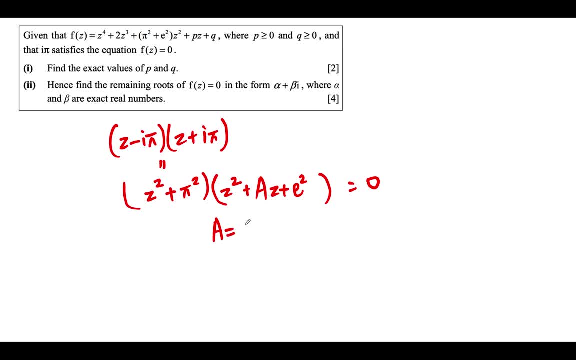 z cube comes from here and it actually is the only place where z cube can come from. so a is 2 right. so we have to solve for z squared plus 2z plus e squared equals to 0, and from here we can just use our either our gc or our quadratic formula. get z equals to minus 2 plus minus. 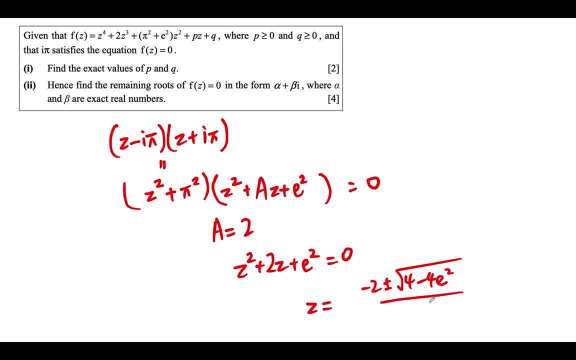 square root 4 minus 4 e squared over 2 equals to minus 1 plus, minus 1 minus e squared. so we have two roots: minus 1 plus square root, 1 minus e squared and minus 1 minus square root of 1 minus e squared. 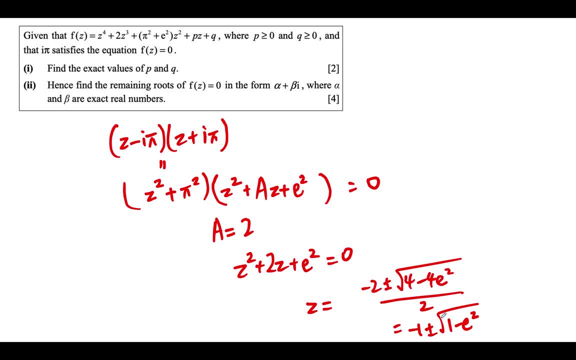 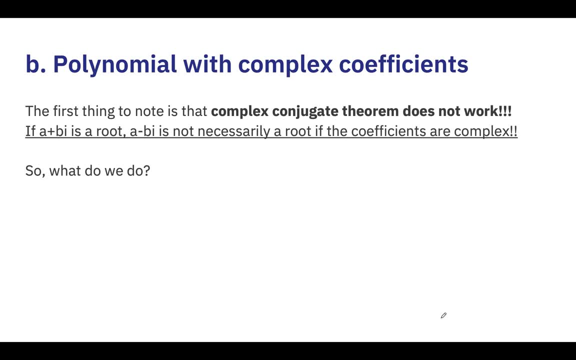 right, so we've completed this question and next we're going to look at polynomials with complex coefficients. okay, this is really important to note that the complex conjugate theorem does not work. okay, when our polynomial doesn't have its coefficients all real and instead it has some complex coefficients. 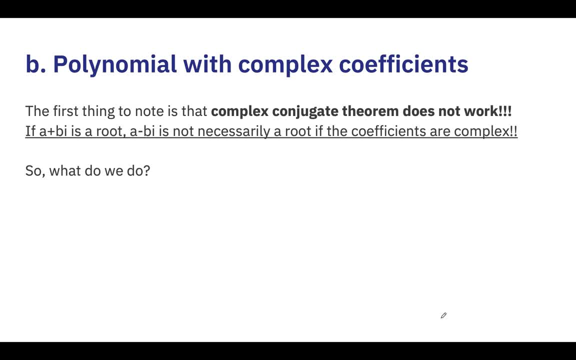 right, so what this means is, if a plus bi is a root, a minus bi isn't necessarily a root if the coefficients are complex. right, so we're going to discuss the techniques involved in solving the various problem types. for example, consider a quadratic equation with complex coefficients. 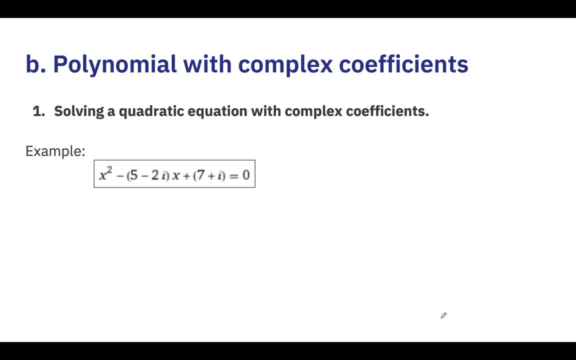 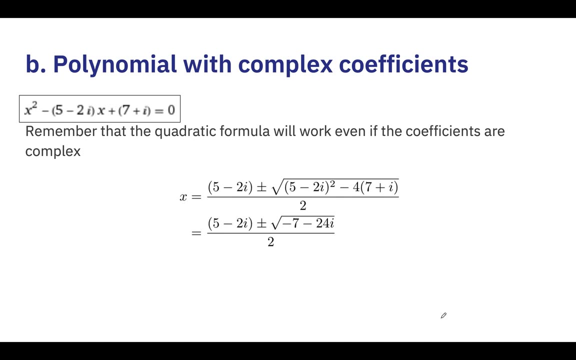 like x squared minus 5 minus 2i, x plus 7 plus i. okay, remember that the quadratic formula will still work, even though the coefficients are complex. it is the complex conjugate theorem that doesn't work right, so we can still substitute it in into the quadratic formula and we'll. 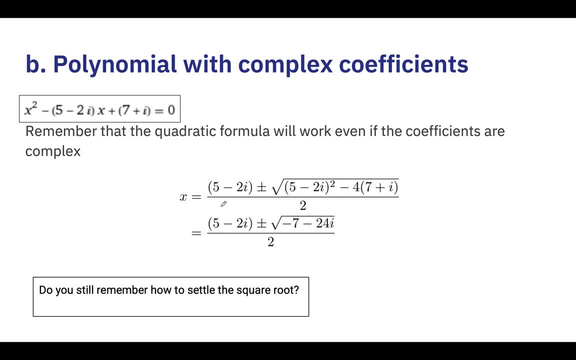 be able to get something like this right. next, we have to learn how to. we have to recall, sorry, how- to settle the square root here, because this can't be our final answer right? we know that this is equals to a complex number that we can express in a rectangular form, but we 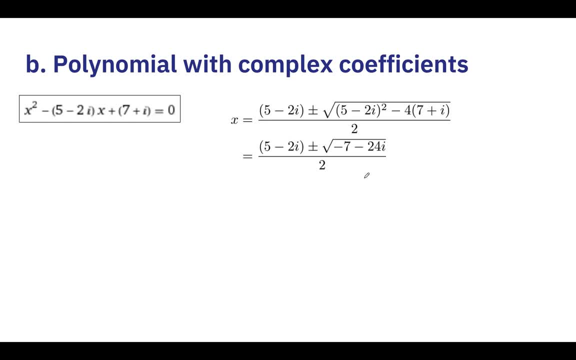 need to be able to express it in the first place. so, in order to do that, we let the square root of minus 7 minus 24i be equals to a plus bi, and then we square both sides. we get a squared minus b squared plus 2abi. next, if we compare: 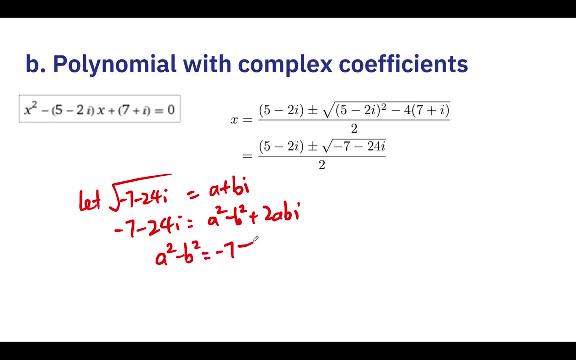 coefficients, we get this: and 2ab equals minus 24, so ab equals to minus 12. right, and solving this using our calculator, we'll get either a equals 3, b equals minus 4, or a equals to minus 3, b equals 4, but either one you decide to, to let it to be the square root, doesn't matter. 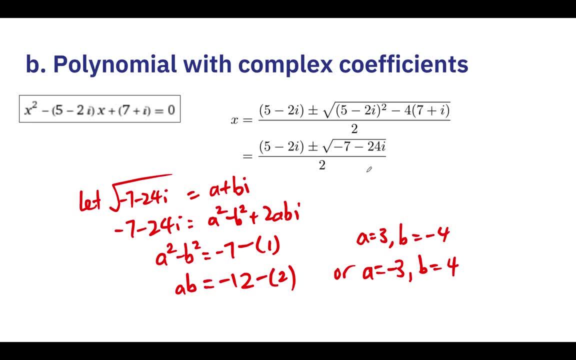 because there's a plus minus sign over here. right, so we will still get two distinct solutions and this set of two solutions are the same for both this and this, so you can use either one of them, okay? next, verifying that a given complex number is a given root of the polynomial. 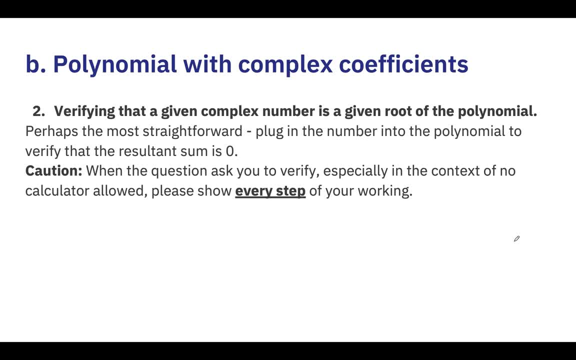 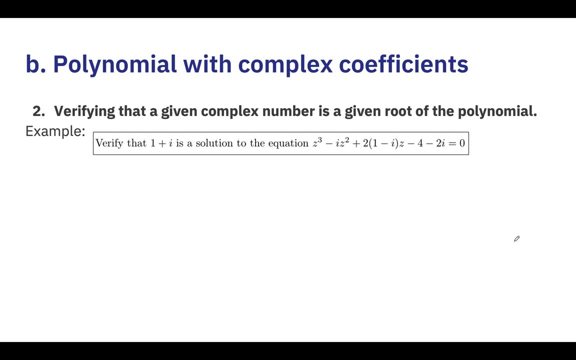 okay. so perhaps the most straightforward way is to plug in the number into the polynomial to verify that the resultant sum is zero. and especially if they say no calculators are allowed, please show every step of your working, okay. so an example would be to verify that 1 plus 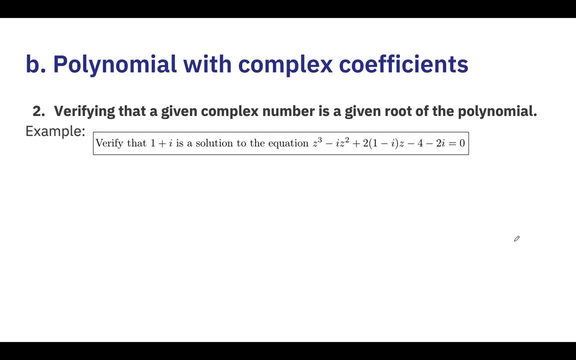 i is a solution to the equation z cubed minus i, z squared plus times one minus i, z minus four minus two i equals zero. okay, so remember to show every step of your working. so what we're going to do is we're just going to substitute it into z right, and we will 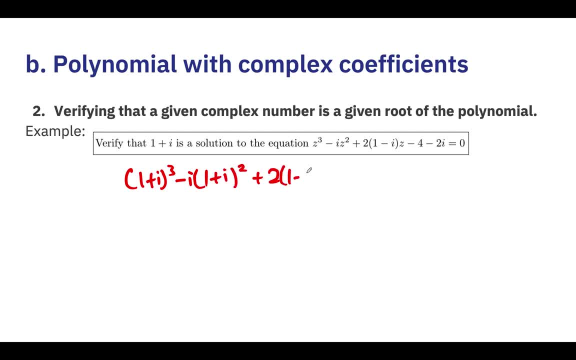 try to simplify this. all right, one plus i. let's do one plus i squared. first, one plus i squared is equals to one minus one plus two i, which is simply equals to two i. and then, when we cube it, we multiply by another one plus i, so it becomes two i minus two. 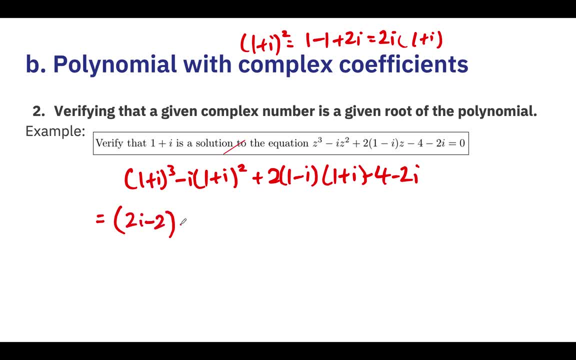 all right, minus i times two i plus two times one minus i. squared, so it's one minus minus one, which is two minus four minus two i. so we get two i minus two plus two plus four minus sorry, plus four minus four minus two i, and we realize that everything. 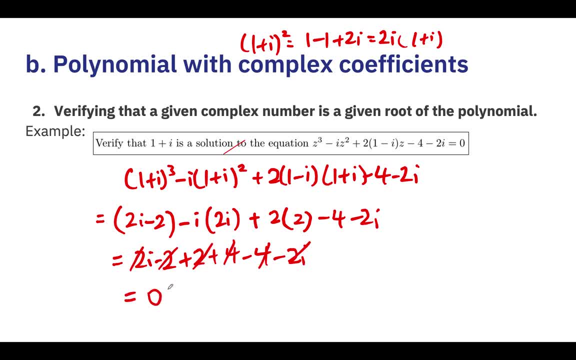 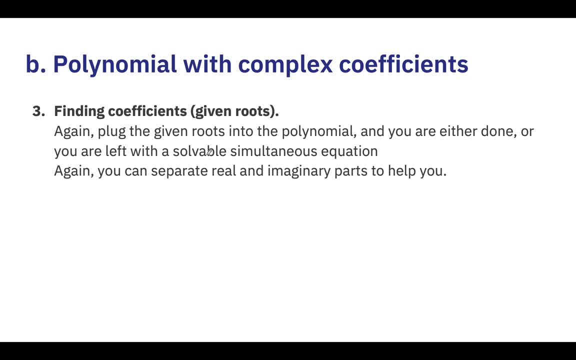 cancels out very nicely to give us zero, and therefore we can verify that one plus i is a solution to the equation. okay, so, last but not least, finding coefficients given the roots. okay, so again, plug the given roots into the polynomial and either you're done or you're left with a. 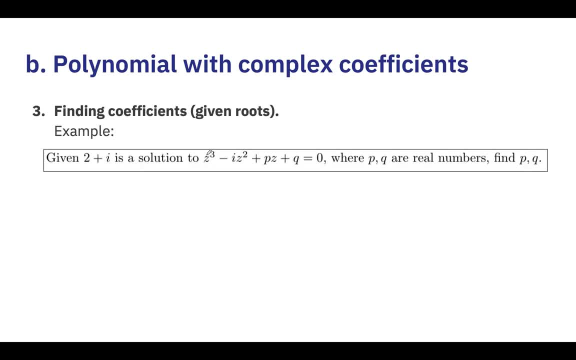 solvable simultaneous equation. so an example would be given: two plus i is a solution, find p and q. so again we're going to substitute it in. and next we want to cube two plus i. so we start with squaring it, of course. two plus i, squared is 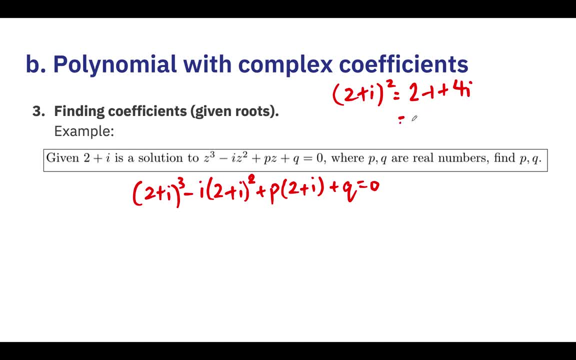 equals to two minus one plus four i equals to one plus four i. then when we multiply this by another two plus i, we will get two plus nine i and then minus four. so we get nine i minus two minus i. times one plus four i plus p. two plus i plus q equals zero, and we try and simplify it more: nine i minus two minus i. 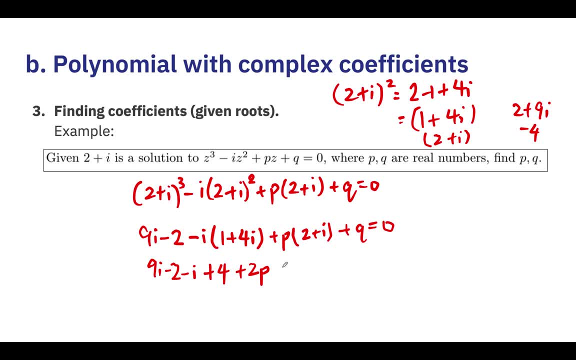 plus four plus two, p plus p, i plus q equals zero. now we solve according to the real and imaginary parts, right? so the real part would be minus two plus four, which is two plus two, p plus q, and then our imaginary part would be nine minus one, eight i, eight plus p. 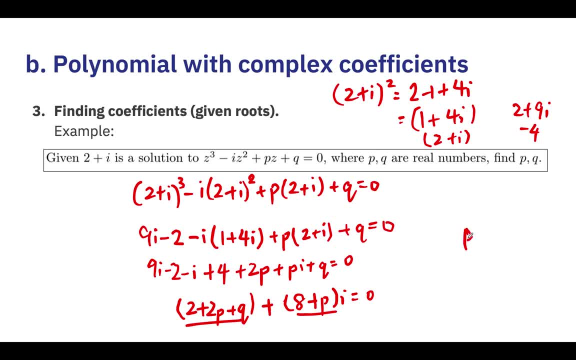 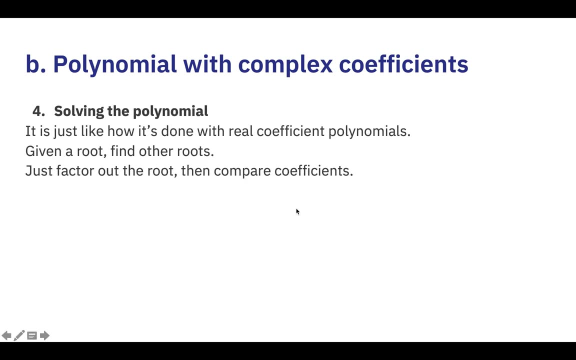 so from here we know that these two are both zero. so p is equals to minus eight, and if we substitute it in here, we get that q is equals to 14.. Alright, so we've been able to solve the equation in this manner. Okay, next we're going to be moving on to solving. 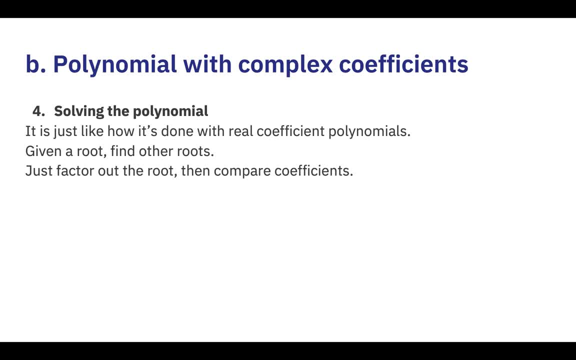 the polynomial. So it is really just like how we do it with real coefficient polynomials: So, given a root, find the other roots. So what we want to do is just to factor out the root and then we can compare coefficients. Alright, so the question says here that, given that z equals minus i is the root of 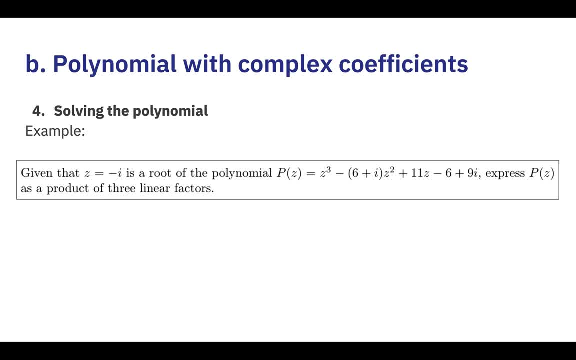 this polynomial over here express pz as a product of three linear factors. So the first thing we want to do is to write out, to factor out, the z equals minus i factor. And to do that we are going to factor out z plus i And then we will have the remaining z squared. 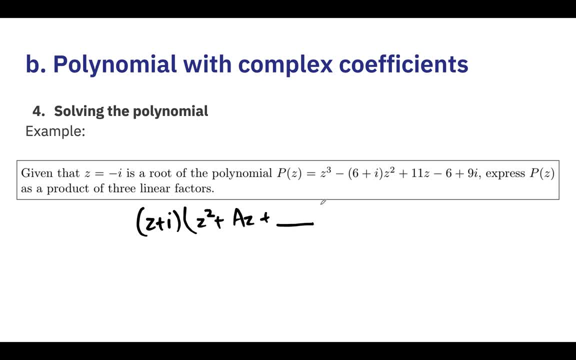 plus az, plus an extra term over here, Alright, and we realize that i, multiplied by this extra term over here, is the only term that will give us a term without x not containing z. So it is equal to minus 6 plus 9i. 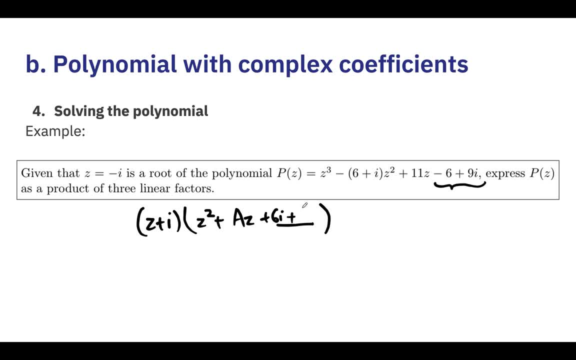 So this thing over here is equal to 6i plus 9.. Because 6i times i equals to minus 6.. 9 times i equals to 9i. And now we simply have to compare the coefficients of z squared. Here, the coefficient of z? squared is a. 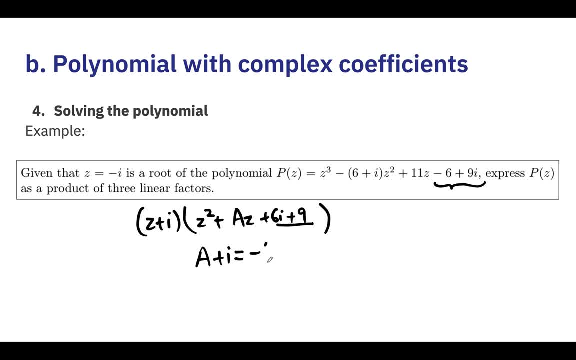 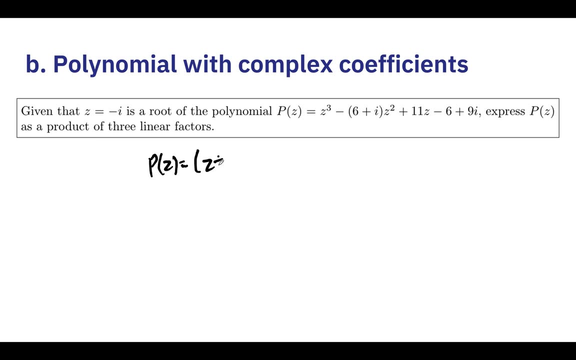 plus i, It is equal to minus 6 plus i. So it is equal to minus 6 minus 2i. So minus of 6 plus 2i. Alright, so we can write pz as equals to z plus i, z squared minus. 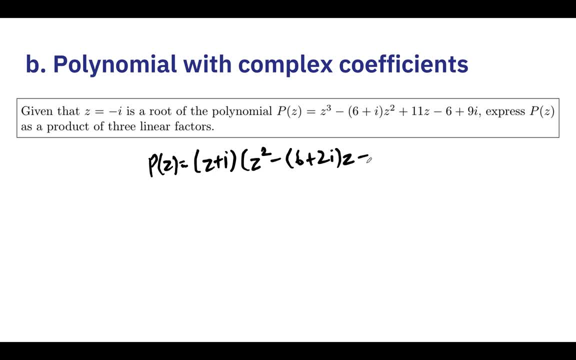 6 plus 2i, z plus 6i plus 9.. Alright, and now we have to read this quadratic to 0 and solve for z. So, in order to do this, we can just use our quadratic formula And we get z equals to 6 plus 2i. 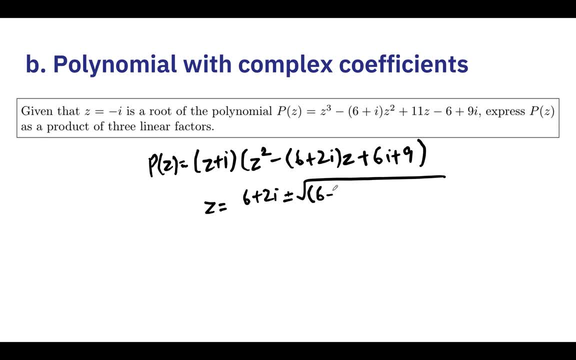 plus minus square root, 6 plus 2i squared minus 4, 1, 6i plus 9 divided by 2.. And if we perform a simple simplification right, this is equals to 36 minus 4, 32 plus 24i minus 24i minus 36 over 2.. And these two terms cancel out. 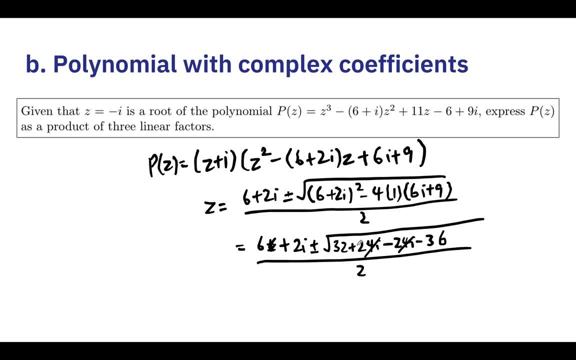 but think: 32 minus 36 on the bottom is equal to minus 4.. And the square root of minus 4 is equal to 2i. So we get 6 plus 2i plus minus 2i over 2.. So either that equals to: 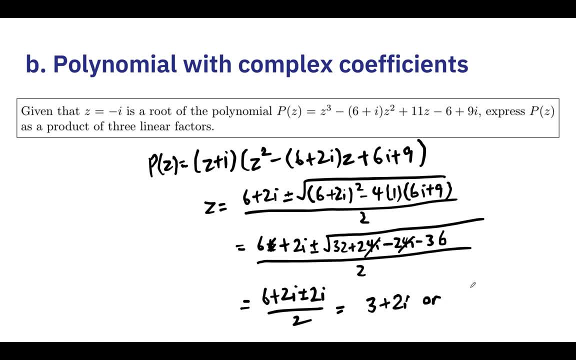 3 plus 2i or 3.. Alright, so we can now express pz as a product of 3 linear factors. we can also cure and get the place of z and root for the lambda of gel molecules. Literally brush your nose. 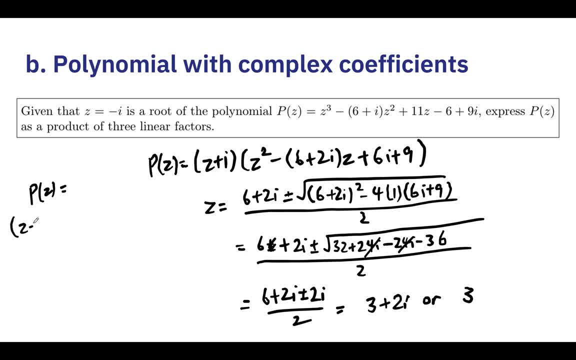 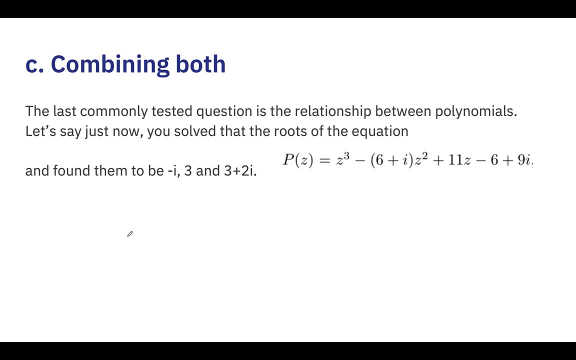 linear factors, pz will be equal to z plus i, z minus 3, z minus 3 plus 2i. just like this, Alright. so the last commonly tested question tests you on the relationship between polynomials, right? So just now we managed to solve the roots of this equation, pz, and we found them to be: 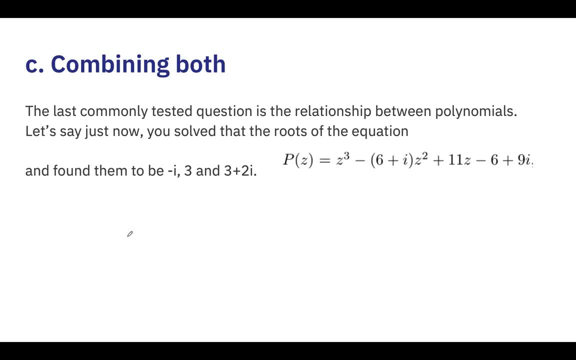 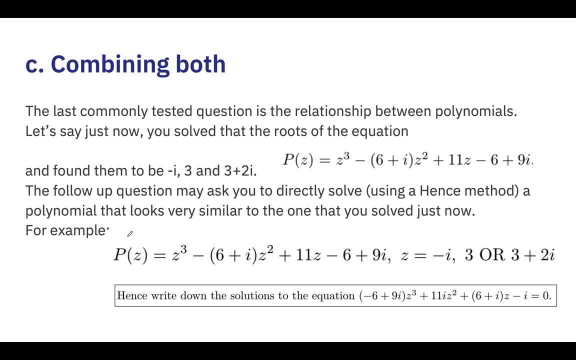 minus i, 3n3 plus 2i. So keep this equation in mind, and a follow-up question for this kind of question may ask you to directly solve, using like kind of a hands method, a polynomial that looks very similar to the one that you solved just now. So it might ask you to hands write down the 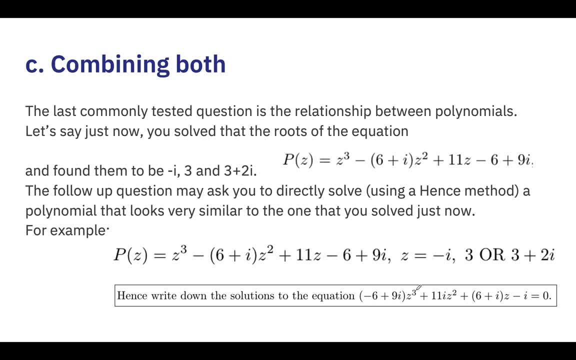 solutions to the equation: minus 6 plus 9iz cubed plus 11iz squared, plus 6 plus iz minus i. So we first need to notice the similarity, because if they ask us for hands, right, then it must be very similar to the previous. 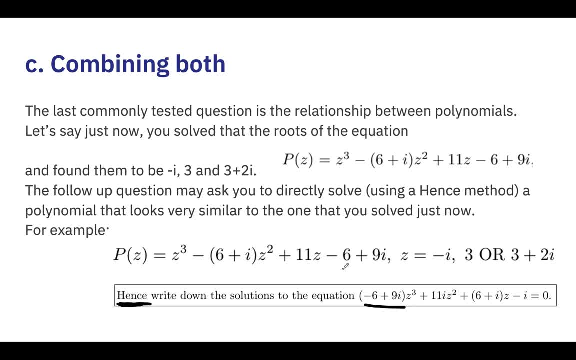 part right. This 6 plus minus 6 plus 9i comes in here, 11 is here, 6 plus i is here. so the structure is kind of the same, but each of these so-called coefficients is paired with a different power of. 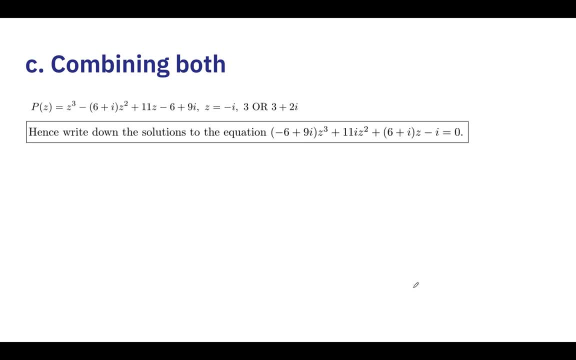 z instead, right? So the trick for this kind of questions is substitution. So what are we going to substitute? So what we have to notice is that the minus 6 plus 9i became an extra. there was an extra z cubed at the. 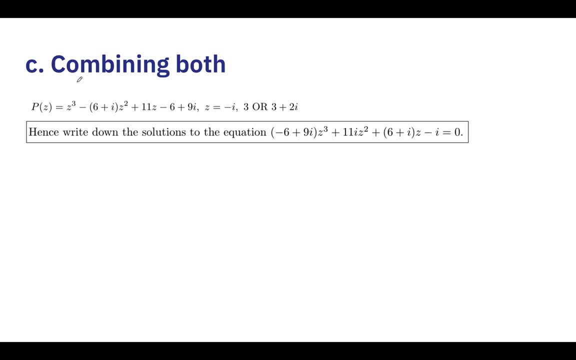 back. So very likely, this entire equation is multiplied by z cubed to go from this term to this term right, And in order to multiply it by z cubed. we can't be keeping this as z cubed here, because if we multiply z cubed by another z cubed, we get z to the power of 6.. Okay so, 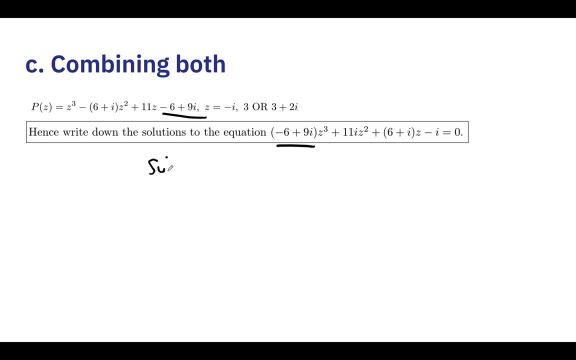 we're going to use the substitution substitute right z goes to i z right. We're going to replace all the z's with sorry, not i z i over z. Okay, we're going to replace all the z's with i over z. 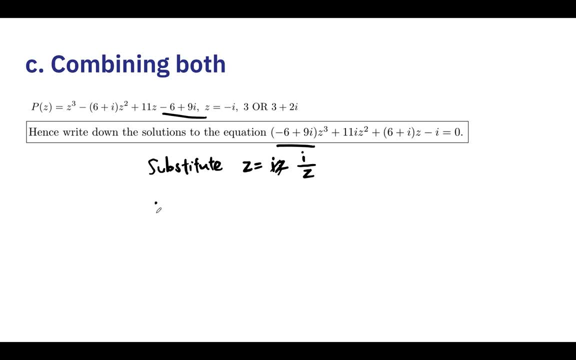 and what happens is we get kind of like a p of i over z equals to i over z cubed minus 6 plus i. i over z squared plus 11 i over z minus 6 plus 9 i Right. and if we were, 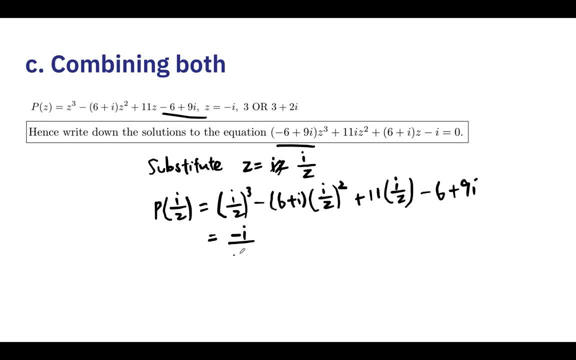 to expand this, we would get a minus i over z cubed plus 6 plus i over z squared, plus 11 i over z accelerate y over z cubed minus 6 plus i over z squared, plus 11 i over z squared. 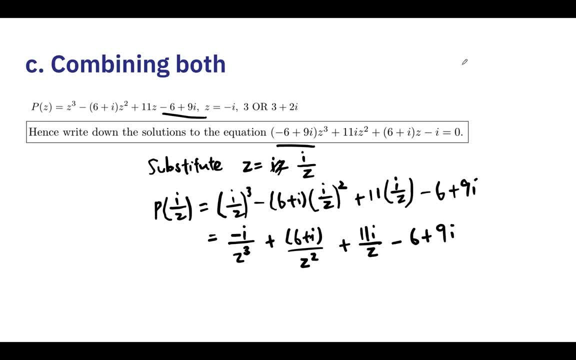 minus six plus nine i, and we want this to be equal to zero, right? so what we can do is we can actually multiply throughout by z cube, because you see, the minus i over z cube becomes minus i, and this term has an extra z cube at the back, so it kind of makes sense to multiply this by z cube. 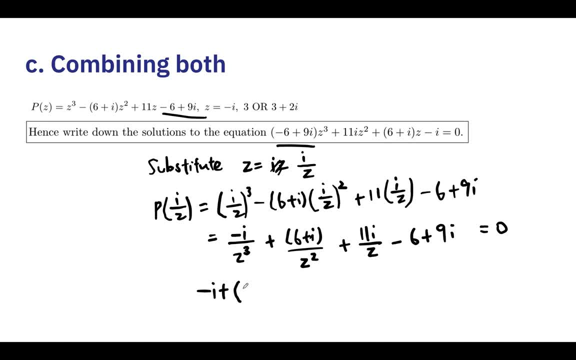 so we get minus i plus six plus i z, because we multiply by z cube. so we cancel out the z square and we add another z plus 11 i z squared minus six plus nine i z cube close to zero. so we realize that we actually have converted this form into this form by simply substituting i over z into. 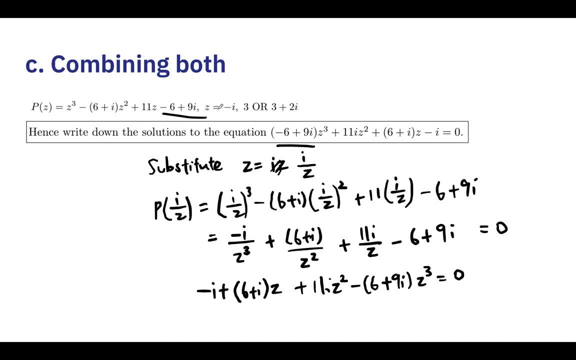 this polynomial over here. so instead of z being equals to minus i, three, or three plus two i, we instead have i over. z equals to minus i, three, i or three plus two, right, right, and then from here we are able to solve for the different values of. 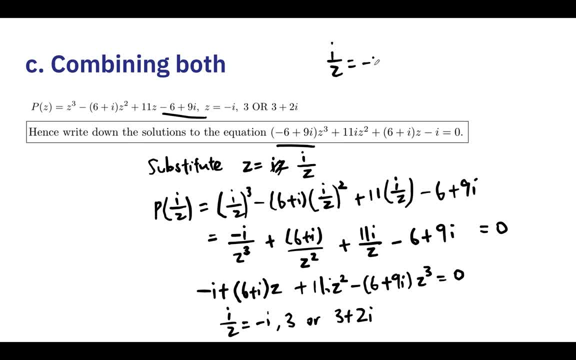 z. so when i over z equals to minus, i, z equals to minus one. when i over three, no, i. over z equals to three, z equals to i over three, or one third i. and last but not least, when i over z equals to three plus two, i. 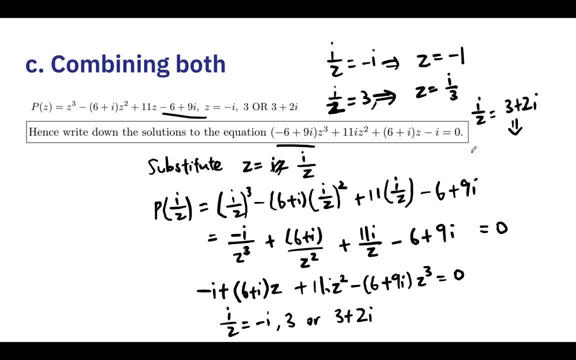 right. then z will be equals to i over three plus two i, and then what we can do here is we can rationalize the denominator right, so i three minus two i, and then the bottom will become three squared plus two squared, which is thirteen. so this becomes three i plus two over thirteen equals to two over thirteen. 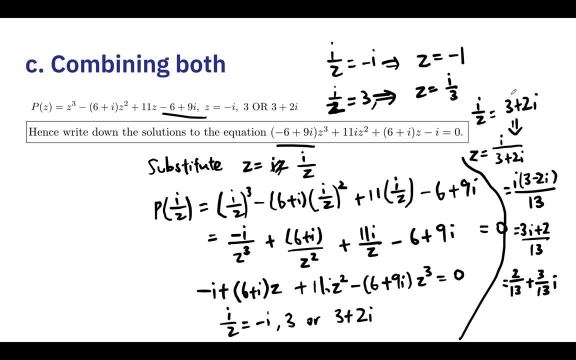 this burton linear par excellence, where z equals to 1 divided by point i, which, kids, is one over point i, is equal to 5 and i is equal to 6. so if we want to rất over this one, this means characters are negative to zero.